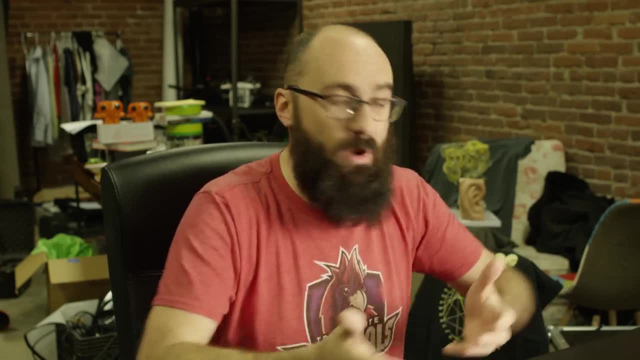 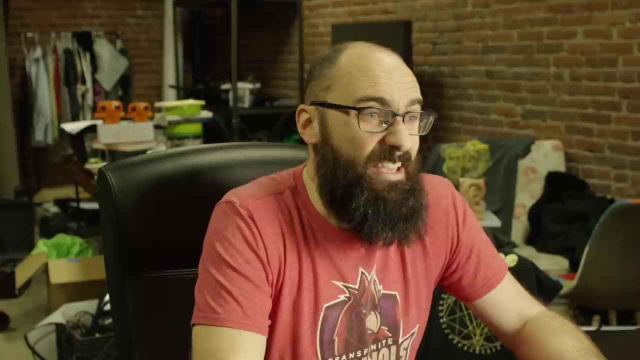 are a lot of fun. They allow us to quite quickly determine whether a given number can be evenly divided by another number, that is, with no remainder left over. Now, a calculator is sometimes faster than these procedures, I'll admit that, But these procedures allow us. 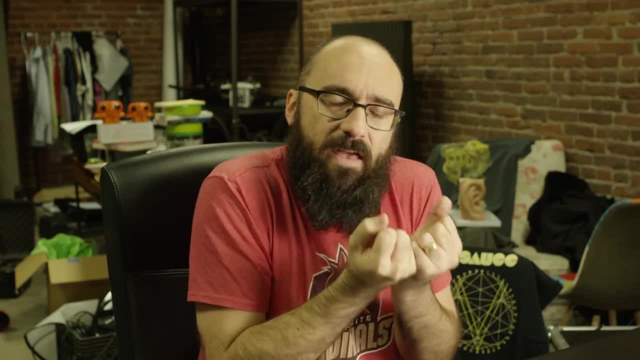 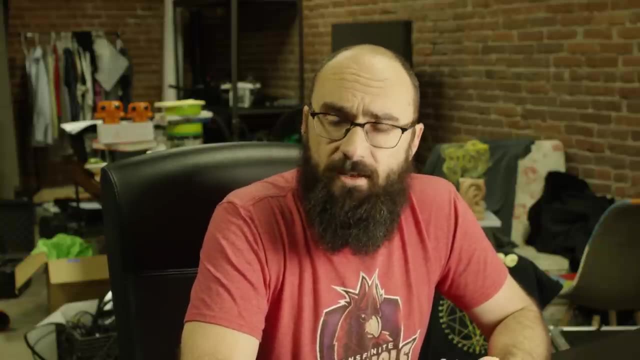 to do two things: They allow us to develop our number sense and they also allow us, in these lonely times, to make a bunch of new friends, Math friends. Let's get started Now. it's pretty easy to check if a number is divisible. 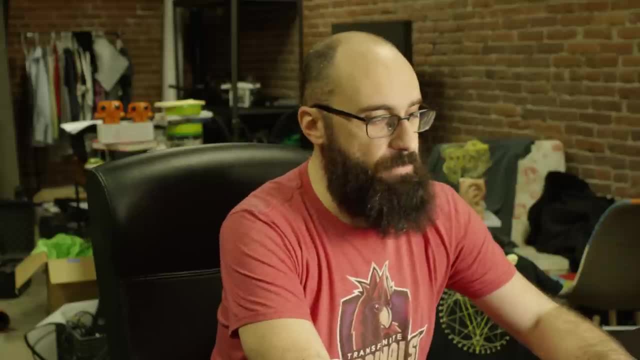 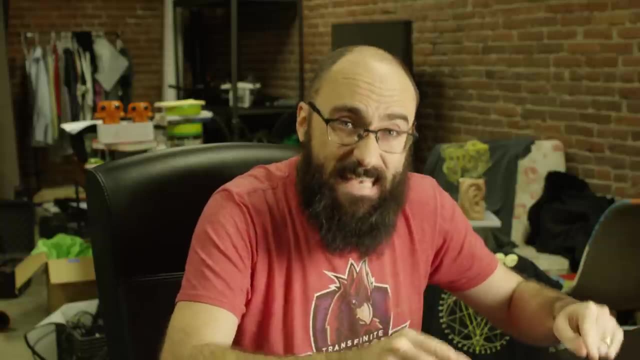 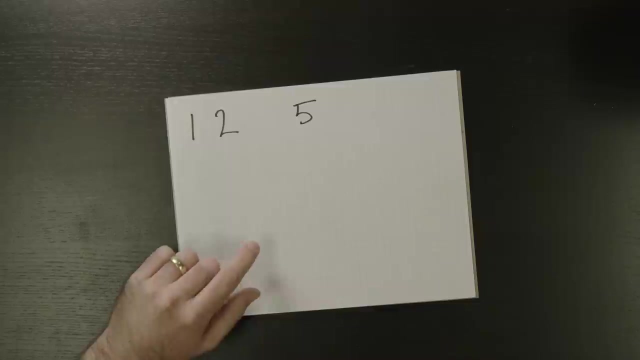 by 1,, 2, or 5.. Because if the number is an integer, if it has no decimal or fractional component, well then it can be divided into groups of 1. If it is even, it's divisible by 2., And if it ends in a 0 or 5, it's divisible by 5.. Now, a lot of us also know a trick for 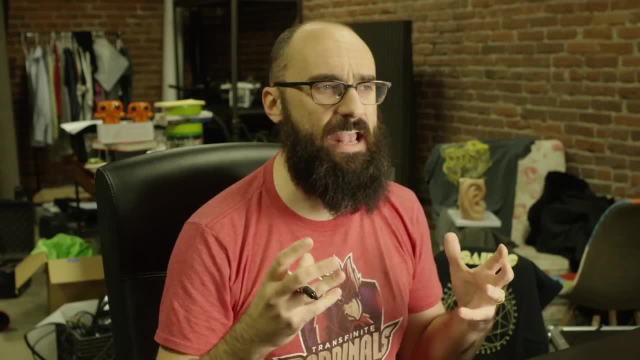 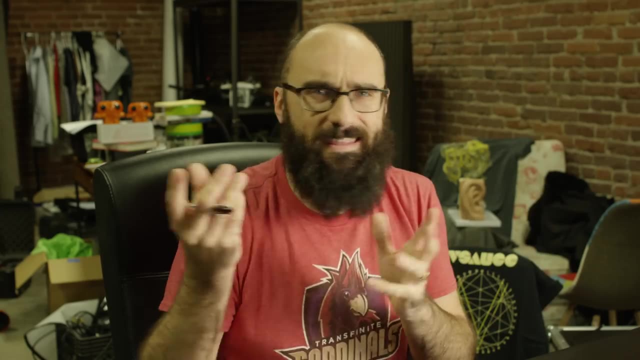 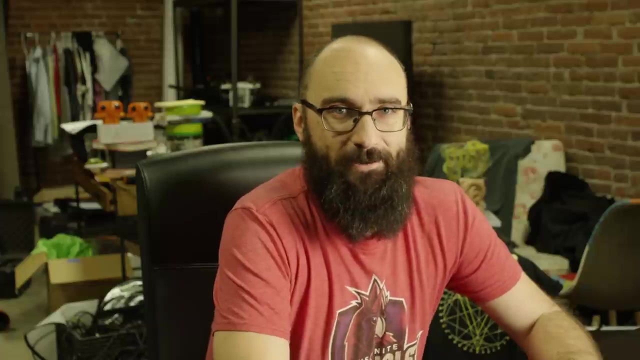 checking divisibility by 3.. The trick is to take all the digits in the given number and if their sum is divisible by 3, so is the actual original number. Let's take a look at this in action. First, let's pick a number completely at random Like: oh, I don't know. 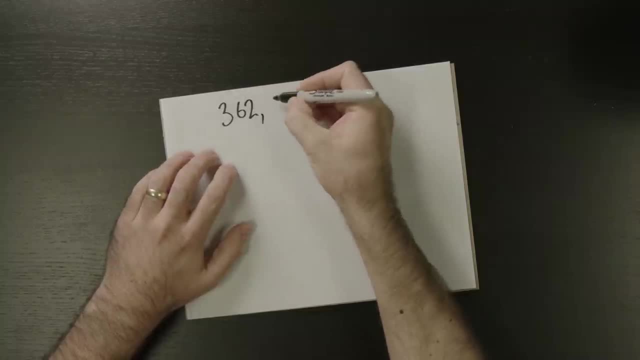 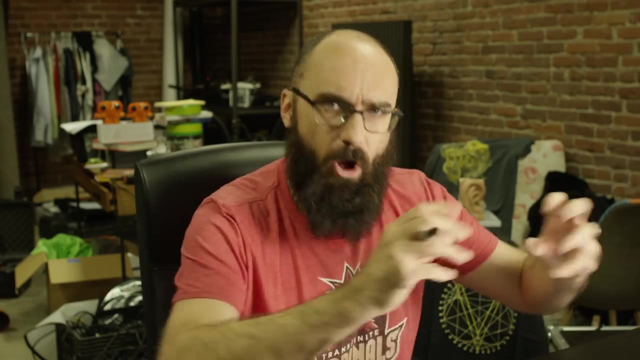 how about 362,880.. Is this number divisible by 3?? Can I take this many things, group them all into 3s and have nothing left over? Well, let's apply our trick. We just simply sum up the digits in the number. 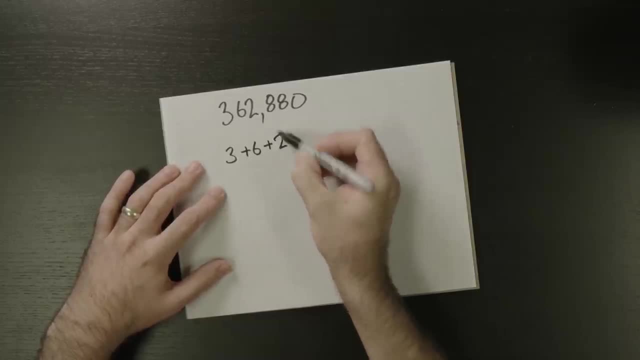 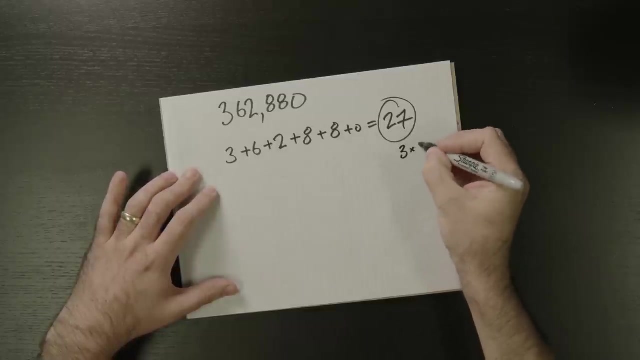 3 plus 6,, which is 9,, plus 2,, which is 11, plus 8,, which is 19, plus 8,, which is 27, plus 0,, which keeps us at 27.. Now, because 27 is divisible by 3,, it happens to be 3 times. 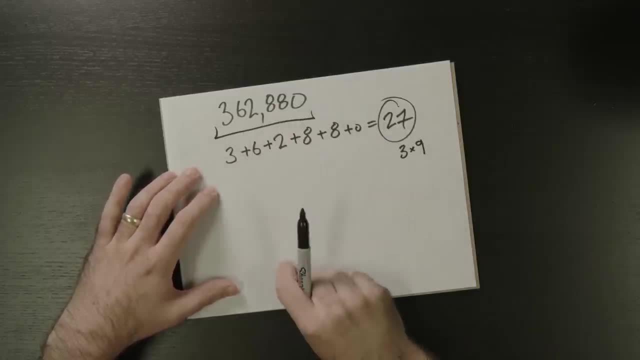 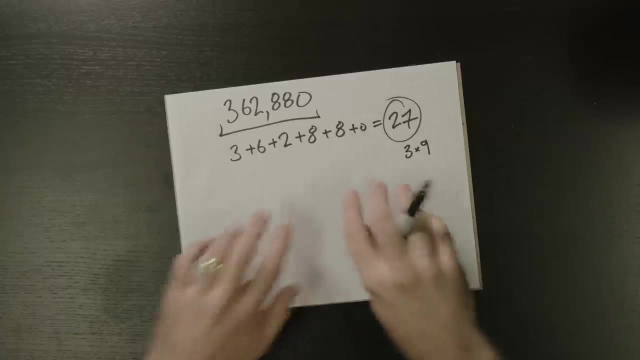 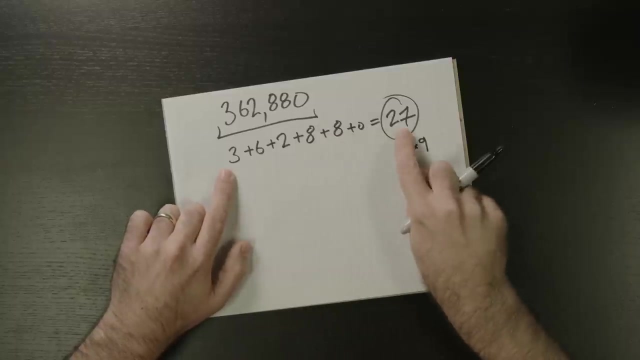 9, so is this original number. So that helps us take care of divisibility by 3.. What about divisibility by 9?? Well, as it turns out, this trick works there too, If the sum of every digit in the spelling of the number sums up to a number, that is. 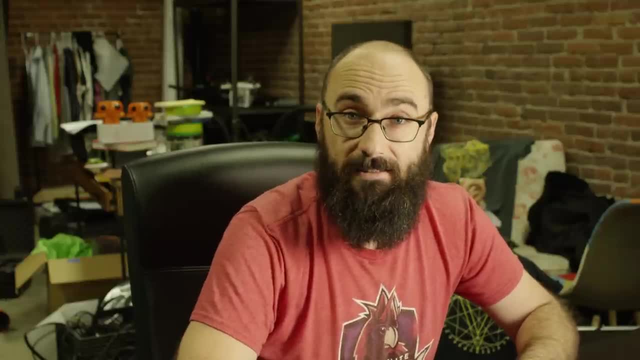 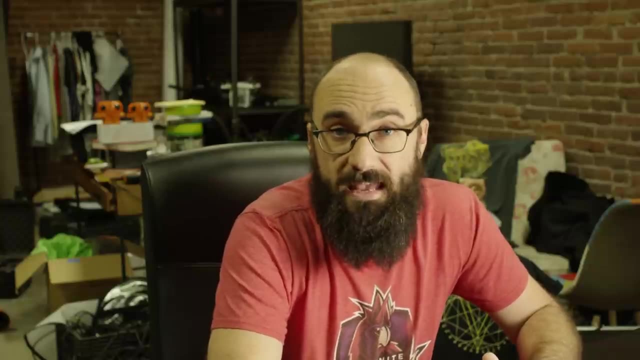 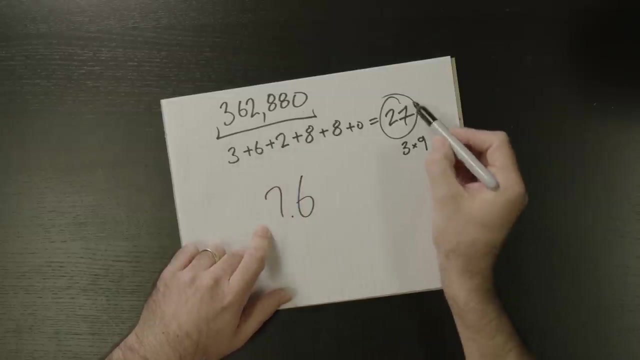 divisible by 9,. well then, the original number is as well. But what about 6?? Well, for 6,, all you need to do is make sure that it is evenly divisible by 3, and that it's even So. in this case, we know that 362,880 is divisible by 3 because this trick shows us that, but 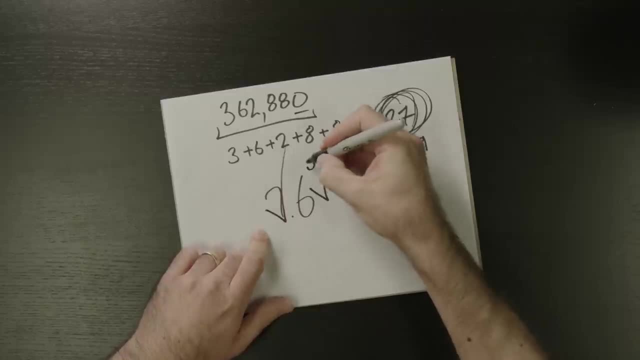 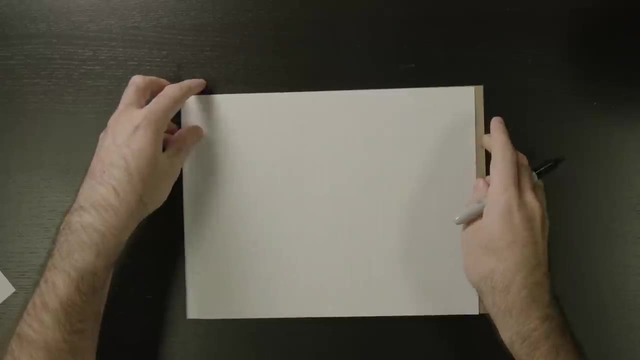 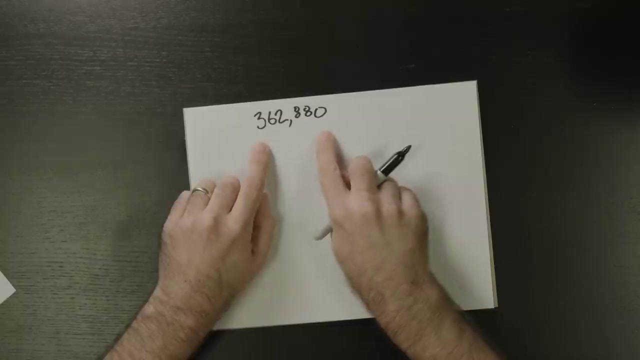 it is also even. Therefore, it is divisible by 6 as well. Subtitles by the Amaraorg community. Okay, now I think it is time for us to move on to divisibility by 4.. We'll keep using the same number: 362,880.. Can I divide this into groups of 4, with no remainder? Well, 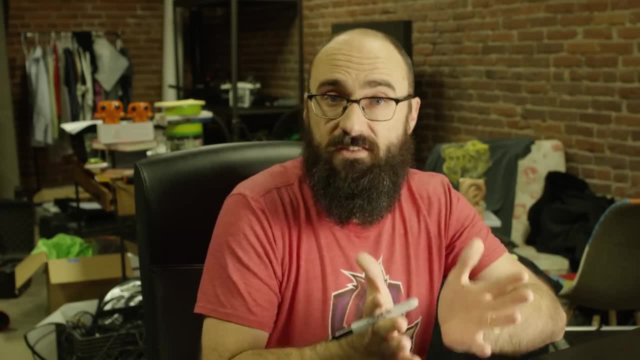 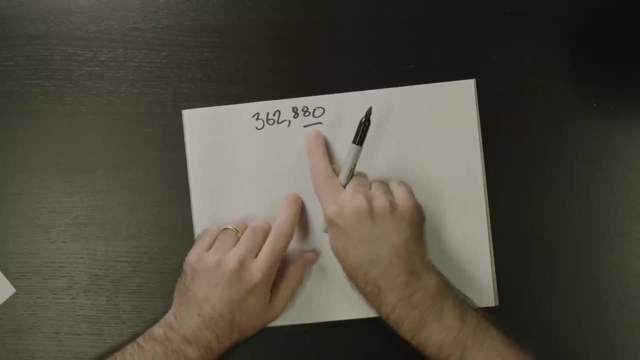 here's how you can check. If the last two digits of a number form a number that is divisible by 4,, then the entire number is. 80 is easily divisible by 4, right, That's just 4 times 20.. 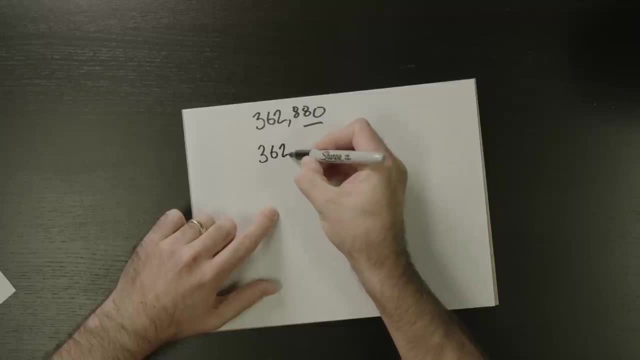 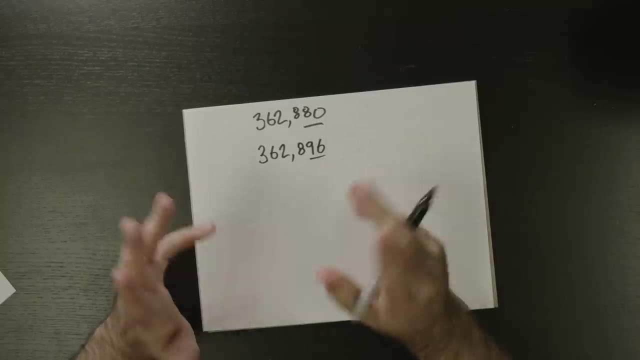 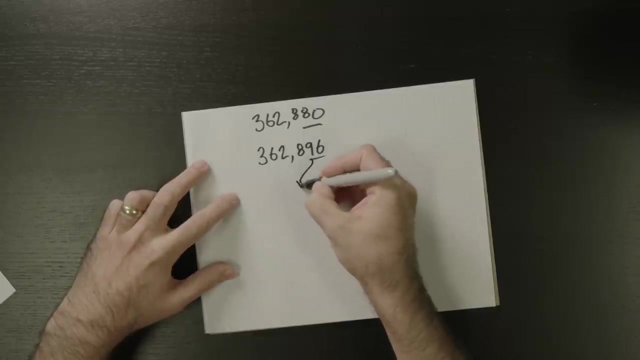 Let's say, though, that we had a different number, like 362,896.. Let's say, I don't know right away whether 96 is divisible by 4.. Well, here's a little bit of a trick you can use to figure out if it is: Simply take the tens digit of this two-digit number and double. 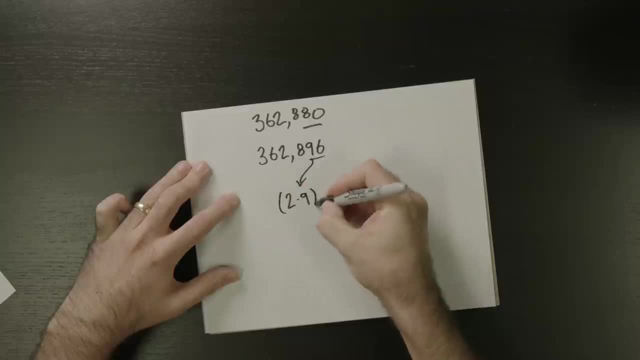 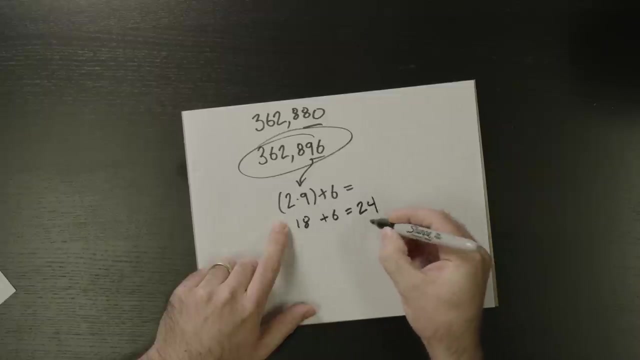 it, which means 2 times 9.. And then add to that the ones digit 6.. If their sum is divisible by 4,, then the original number is 6.. Subtitles by the Amaraorg community as well. In this case we have 2 times 9,, which is 18, plus 6.. This gives us 24, and 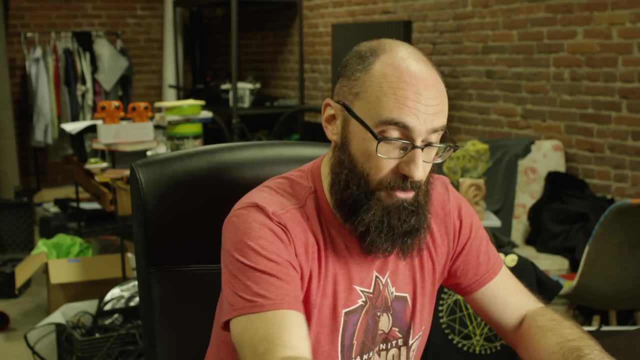 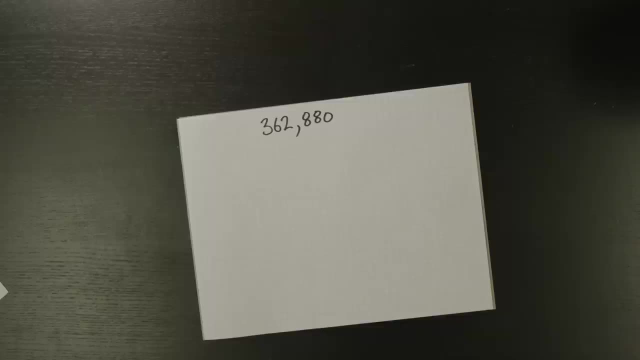 24 is divisible by 4.. So both our original number and this new one can be divided into groups of 4 with no remainder. Pretty cool. What about 8?? Well, if I want to know if a number can be divided evenly by 8, I need to look not at the last two digits but at 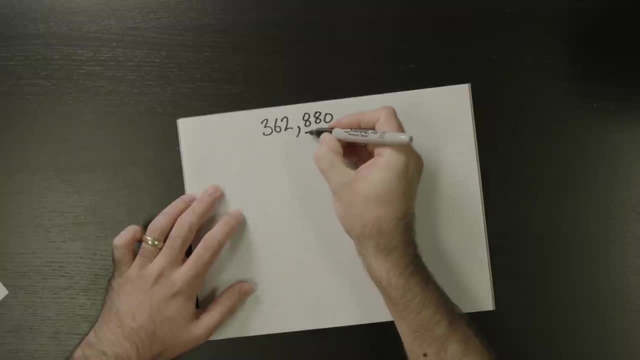 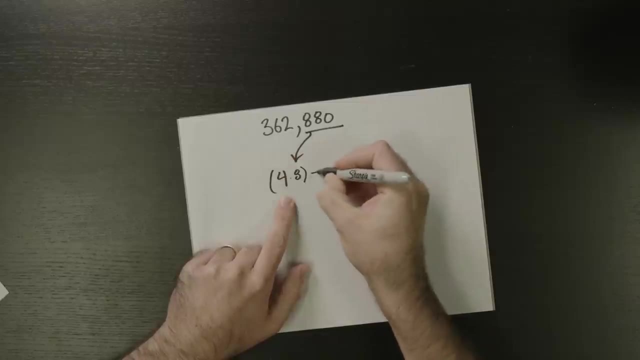 the last three. Here's what I do: I take the hundreds digit and I multiply it by 4. So this is 4 times 8.. To that I add the tens digit times 2.. The tens digit is 8.. 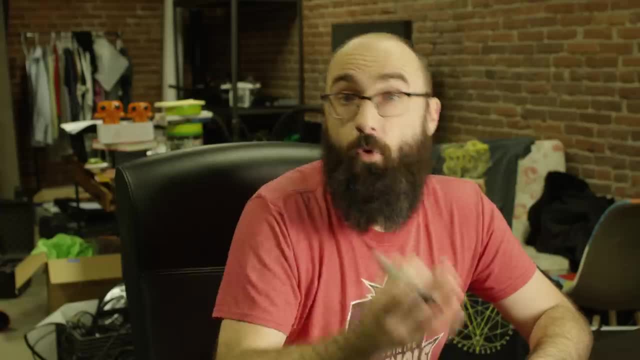 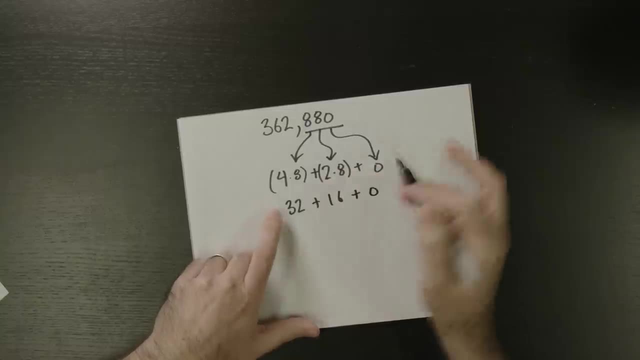 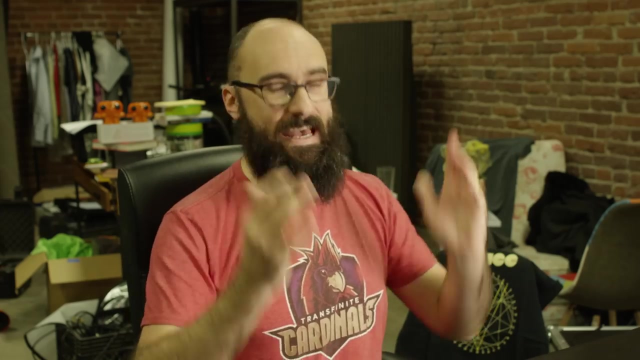 And then to that I add the ones digit 0. 4 times 8 is 32.. 2 times 8 is 16.. And 0 is just 0. Now 32 plus 16 is 48. Is 48 divisible by 8? Yes, it is. It happens to be equal to. 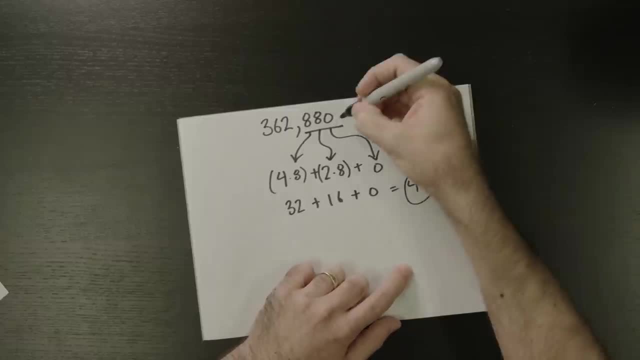 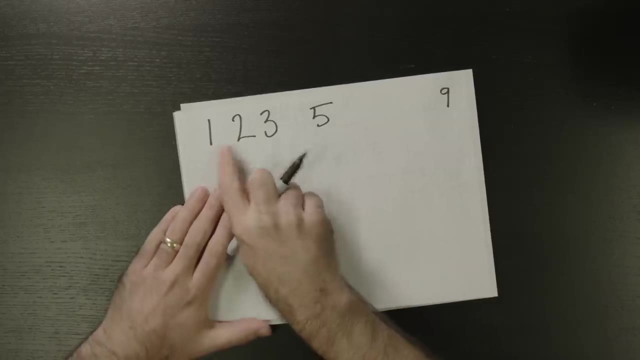 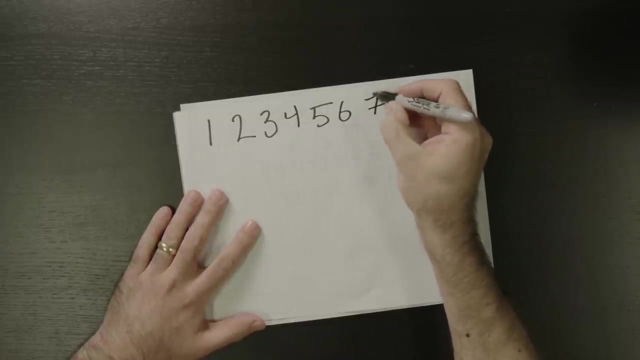 8. 8 times 6. So our original number is evenly divisible by 8.. Okay, so we have covered divisibility by 1, 2, 3.. We've done 4 and 5 and 6 and 8 and 9.. Ho ho, ho. What about 7?? Well, 7 is. 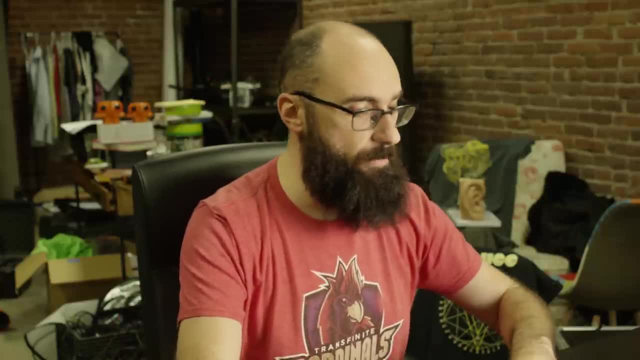 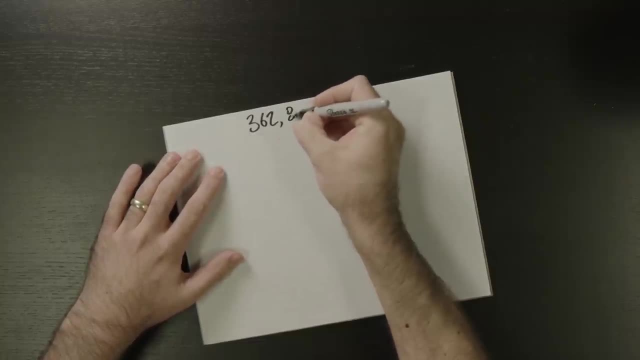 very, very fun. Here's what you do with 7.. I think that for a number as long as our starting number, which has 6 digits, we're going to probably have to do this procedure multiple times. But all of these tricks can just be done repeatedly. You just do it once. 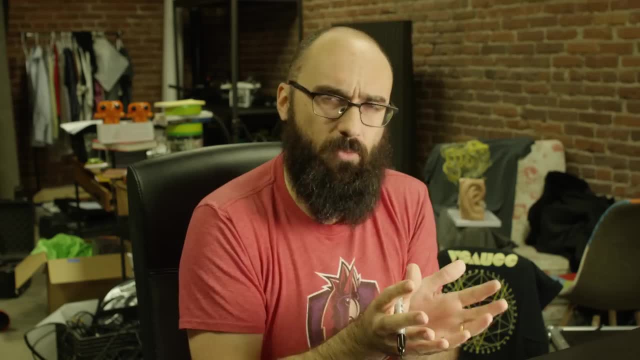 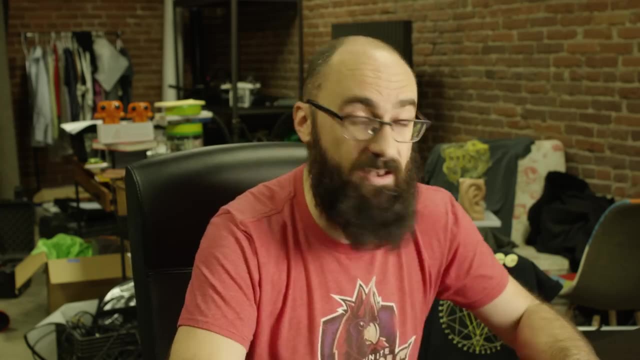 to the original number And then, if you still don't quite recognize what you're left with, and whether it's divisible by the target number or not, guess what- Just keep applying the trick until you see something you recognize. We're going to definitely have to do that. 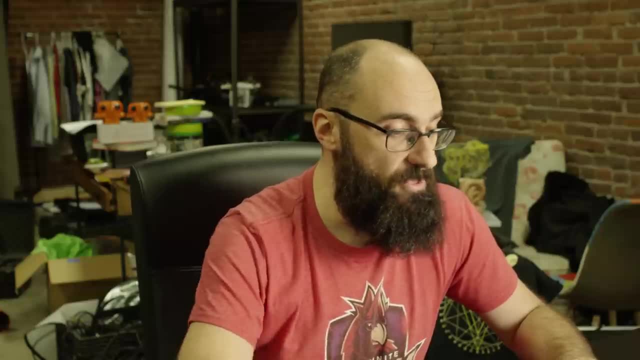 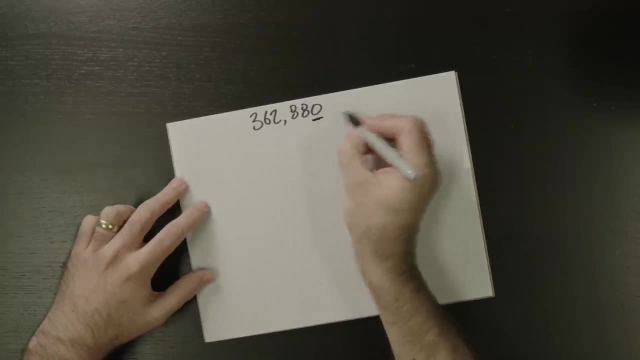 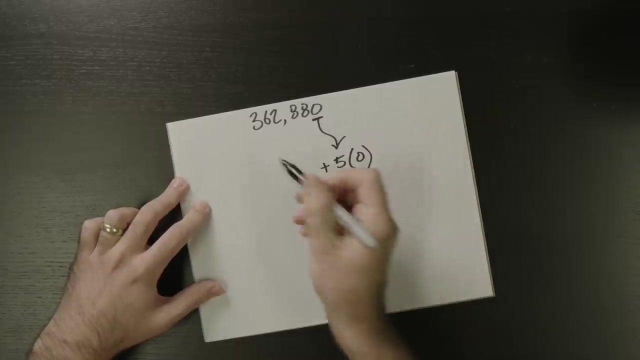 when we check divisibility by 7 for 362,880.. But here's all you have to do: Take a look at the number and look at the ones digit, Apply it by 5,, okay, And then add to this what's left, as if it's a number all by itself. 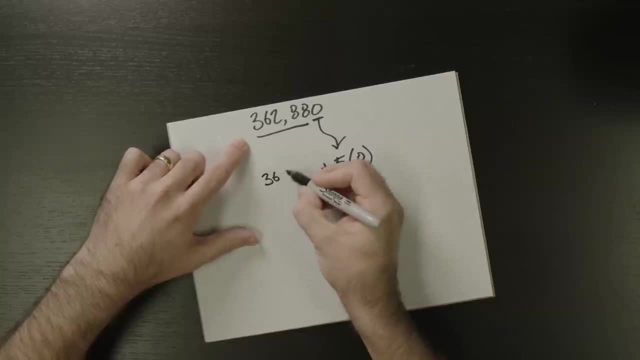 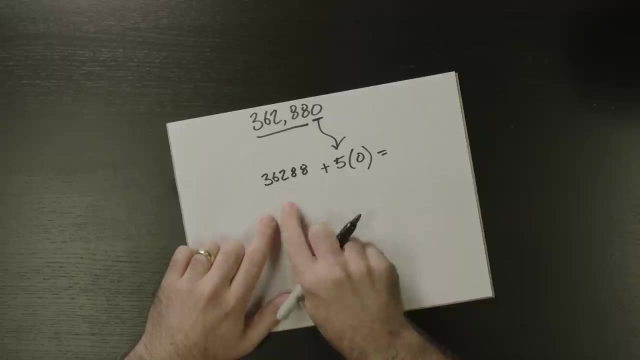 which means we're going to add 5 times 0 to 36288.. All right, Now we sum these up, And if their sum is divisible by 7, then the original number is as well. So what do we got here? 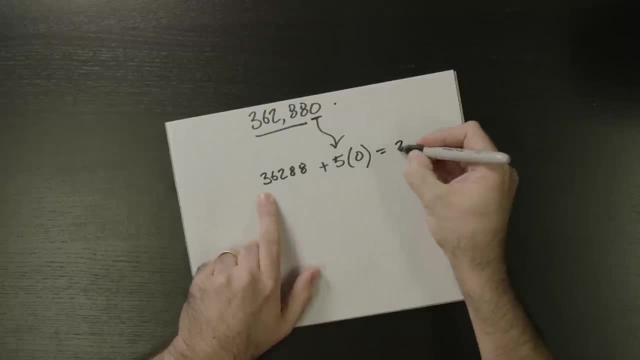 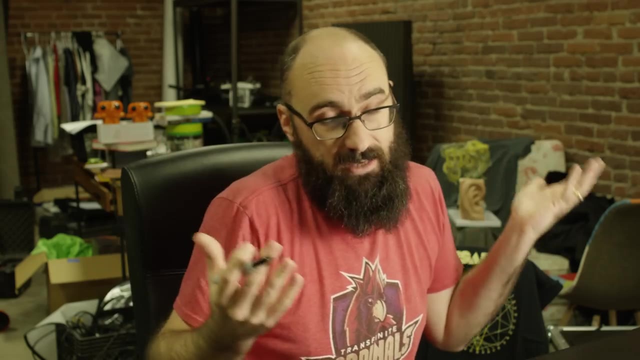 Well, we've got this number plus 5 times 0, which is 0. So it's just the same number. Now I'll be honest, I'll admit this. I'm not afraid to. I don't know if this is divisible by 7 or not. Actually, I do, because it's not a coincidence. 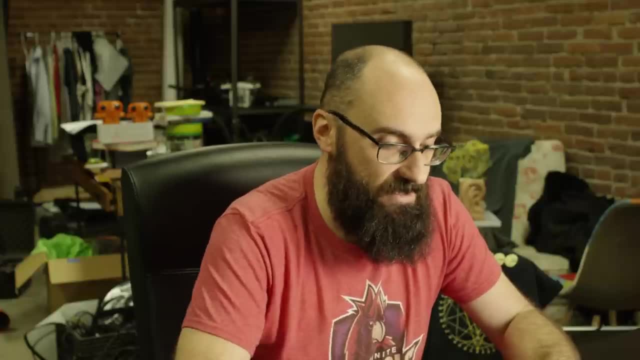 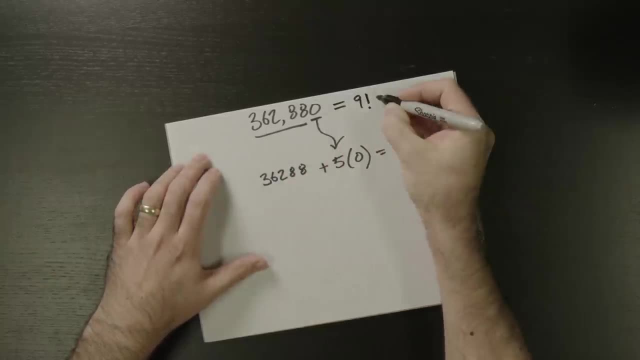 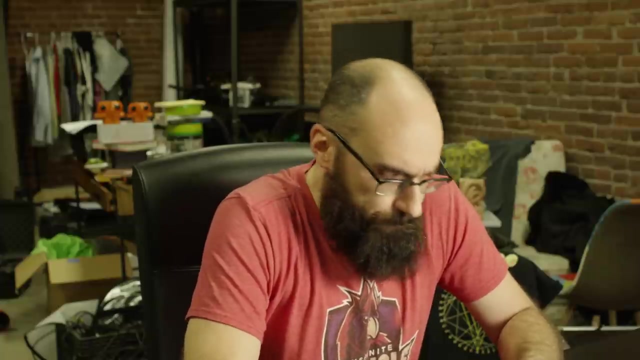 that literally every single one of these digits evenly goes into this number. 362880 happens to be 9 factorial, which means it is equal to 1 times 2 times 3 times 4 times 5 times 6 times, 7 times 8 times 9.. Therefore, it is a multiple of all of them. 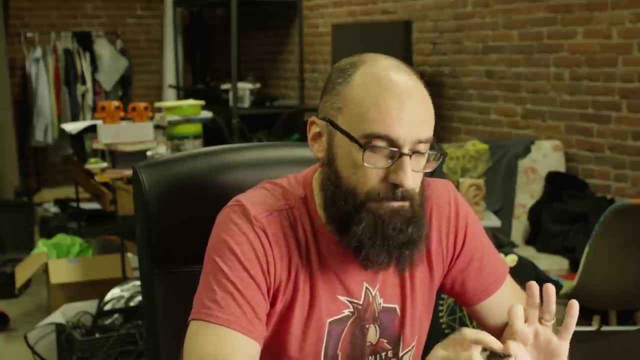 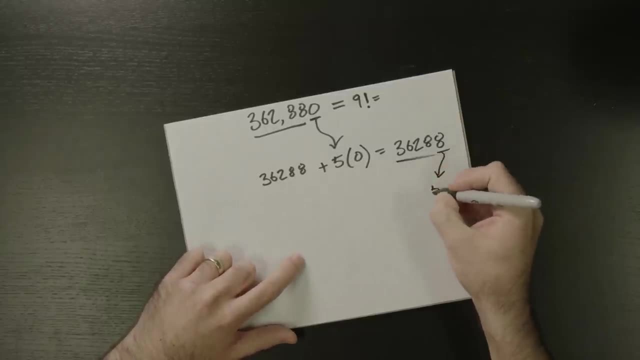 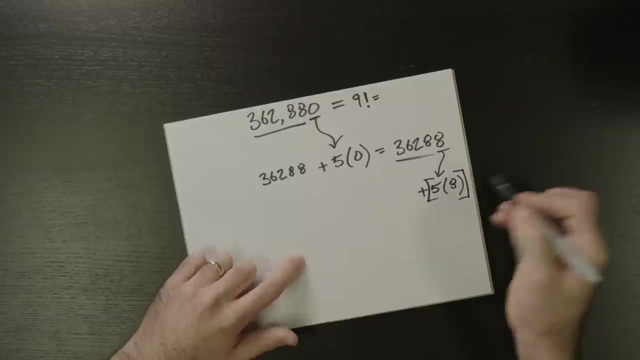 But let's show that, using this trick, I can apply the trick again to the result here. All that means I need to do is I take the ones digit, I multiply it by 5.. So that's 5 times 8.. And then I add to this expression what's left, which is just 3628.. Now 5 times. 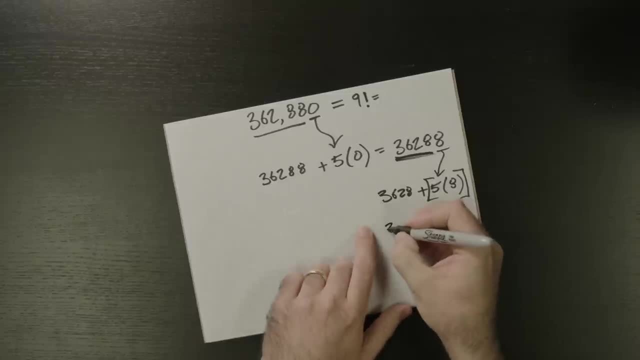 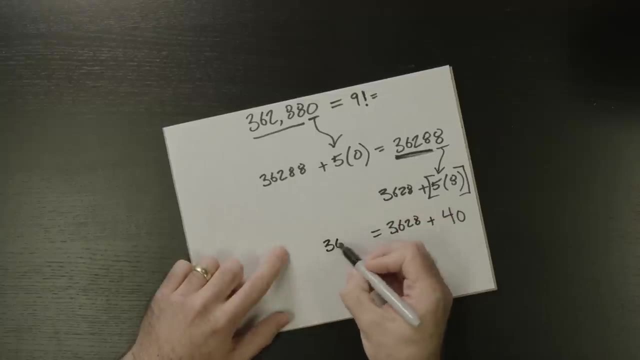 8 is equal to 40. And this number is 3628.. If I sum them together, what I get is 3668.. All right, All right. If I still don't know if this is divisible by 7, I just keep going. So we take the ones. 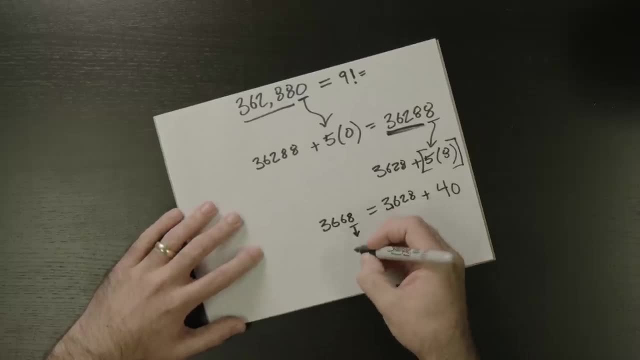 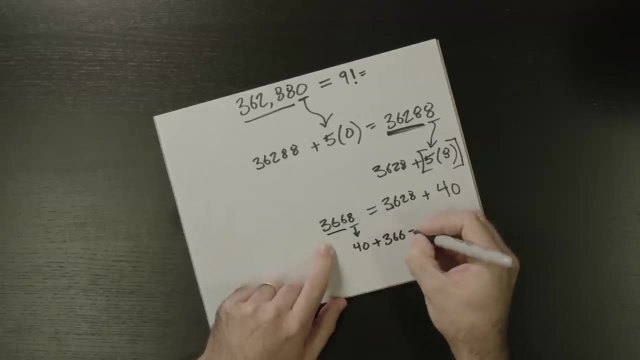 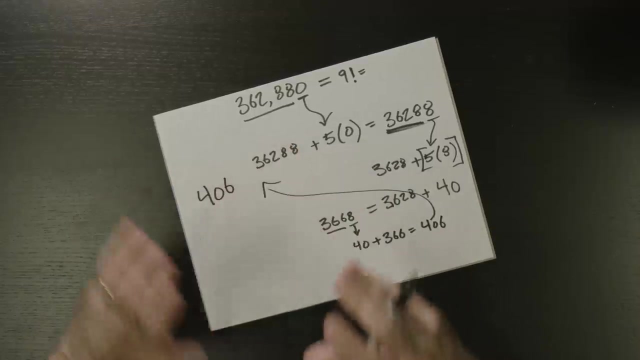 digit, all right, and we multiply it by 5.. 8 times 5, again, as we know, is 40. And then I add what's left: 366.. Okay, This gives us 406.. Is 406 divisible by 7?? If I still don't. 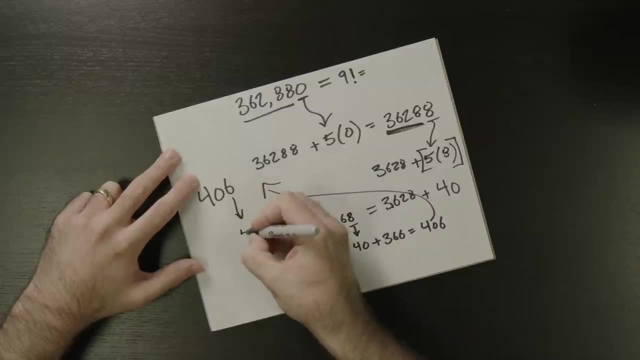 know we just keep going. What is 6 times 5?? Well, we'll deal with that later. We just know that we need to take 5 times the ones digit and sum it with what's left: 40. Now. 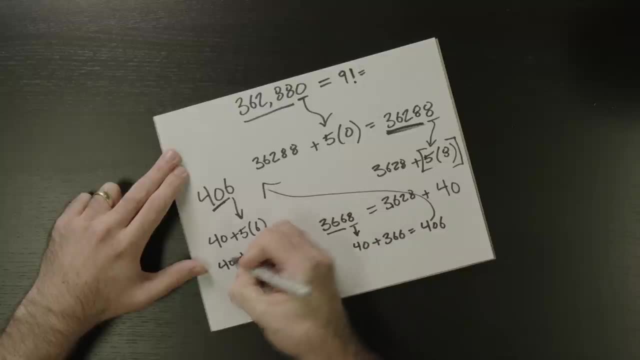 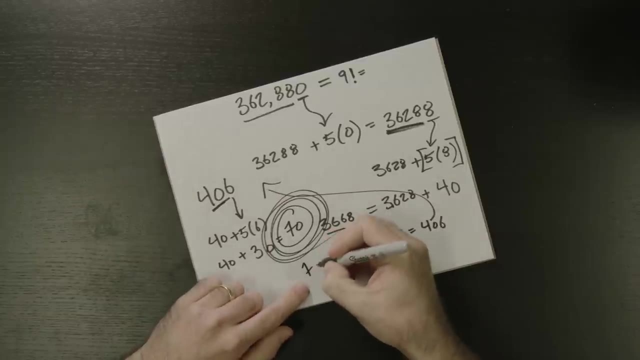 5 times 6 is 30. And 30 plus 40 is 70.. 70, I easily recognize as being divisible by 7.. It is just 7 times 10.. Therefore, because this is divisible by 7, our original number. 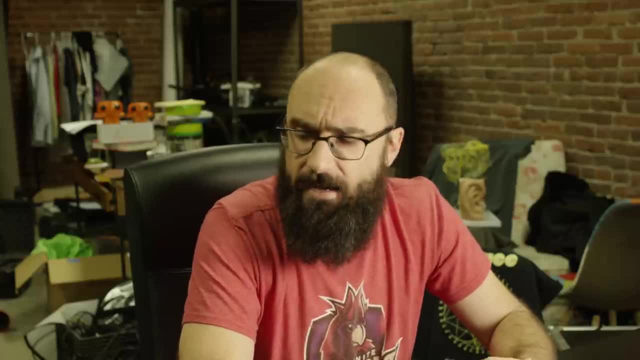 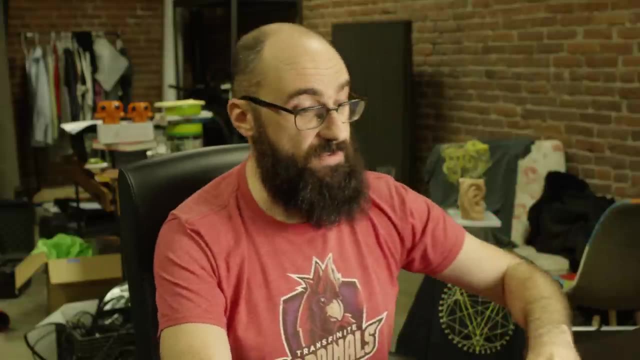 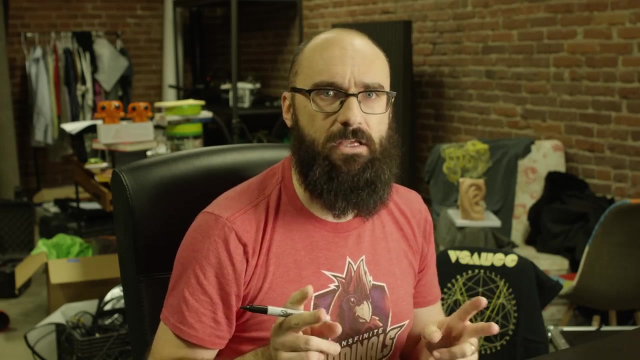 is 2.. Pretty cool, Very fun. But how do these tricks work? Oh well, that's the fun part, Let's get into it. Let's start with divisibility by 3.. Why should it be the case that summing all of the digits used in the spelling of a number 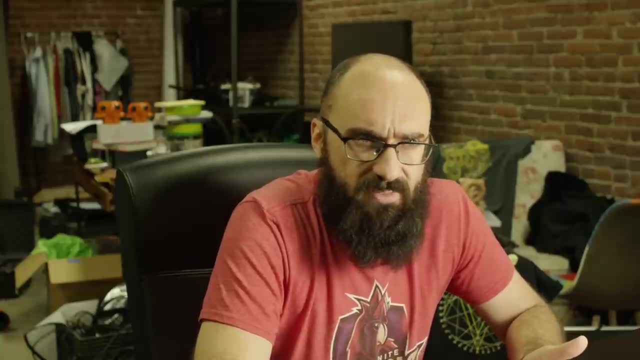 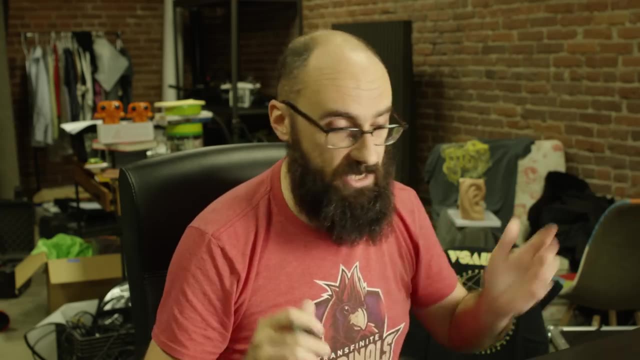 and then checking if that sum is divisible by 3 tells us anything about the divisibility by 3 of the original number. Well, let's generalize this and just imagine a number that has, let's say, three digits. This works for a number with any number of digits, though, But let's 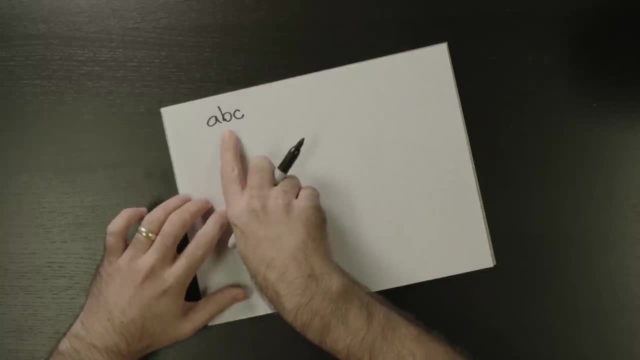 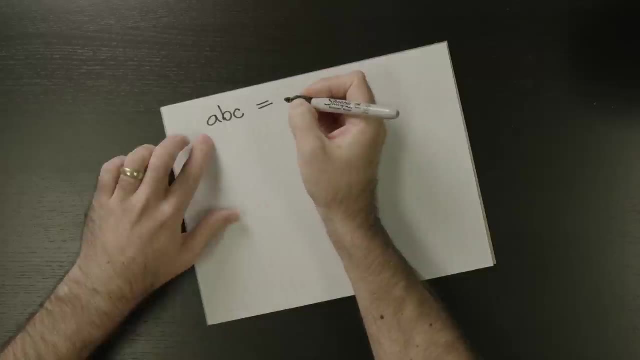 digit number a, b, c, where a is the hundreds digit, b is the tens digit and c is the units digit. Now what a b c means? when we write it down we don't actually mean: yeah, a b c. 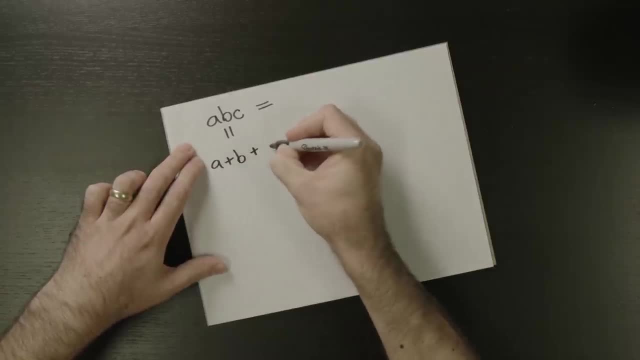 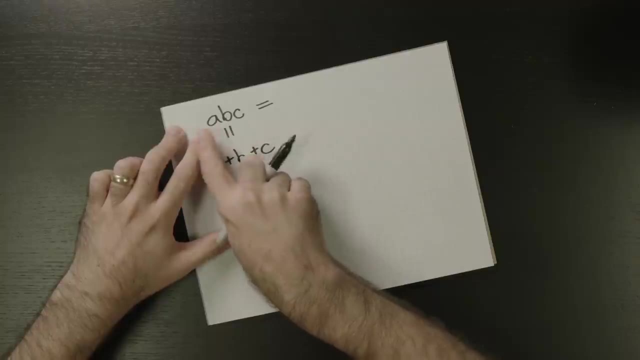 That means you know a number of things equal to a plus b plus c. No, no, no, no, no. Instead, we use a base 10 positional system, where this actually means 100 times a plus 10 times b. 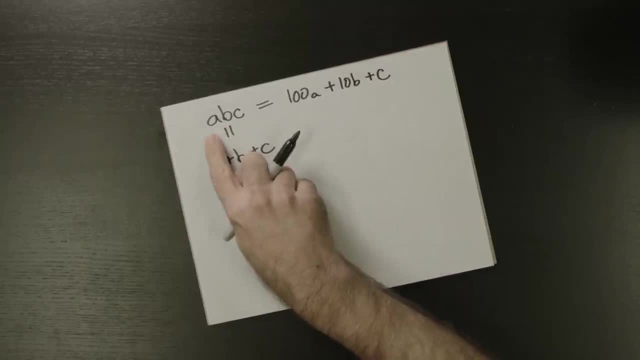 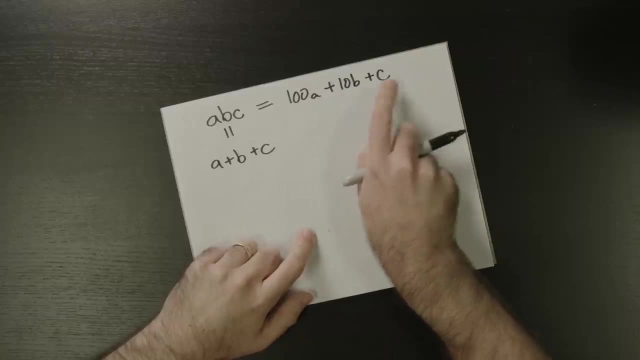 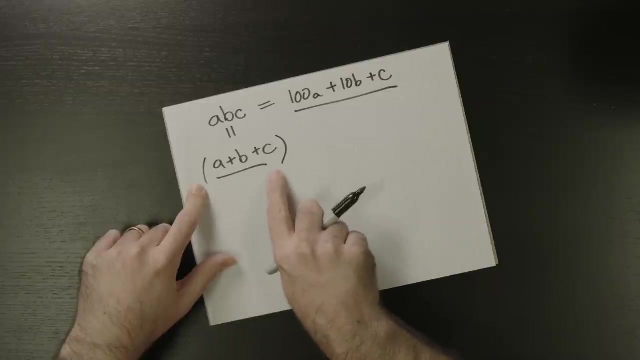 plus c. So if this number is, say, 417,, well then we're going to have four 100s, one 10, and seven units. But let me ask you this: What would it take for this, the sum of the digits in the number, to equal the actual amount the number represents? 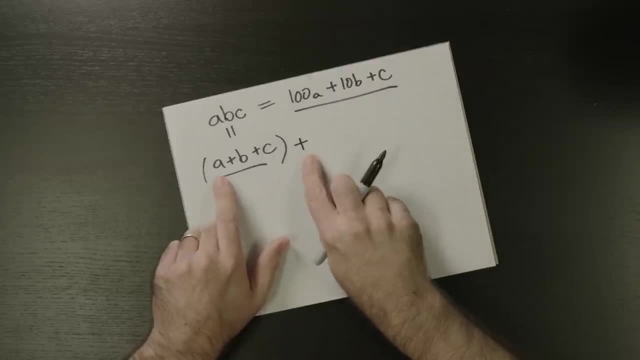 Well, we'd have to add more stuff to this. We only have one a here, but we need 100.. So we're going to have to add more stuff to this. We only have one a here, but we need 100.. 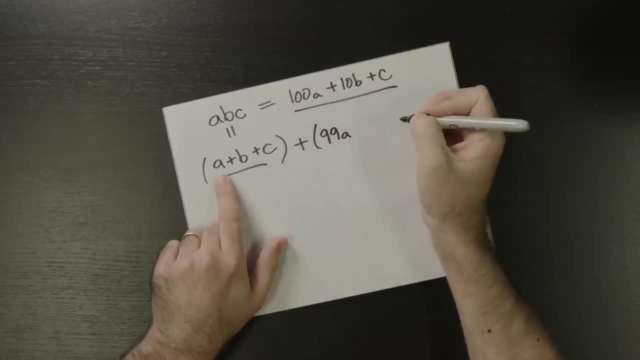 So we're going to have to add more stuff to this. We only have one a here, but we need 100.. So we're going to need 99 more a's, And we only have one b, but we need 10.. So that means we're. 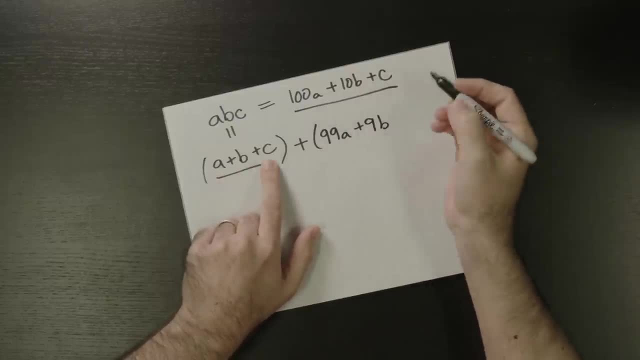 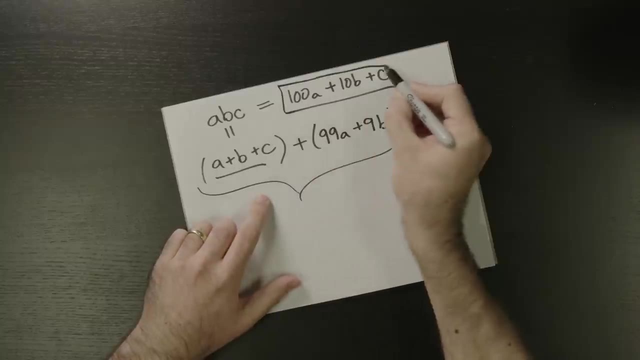 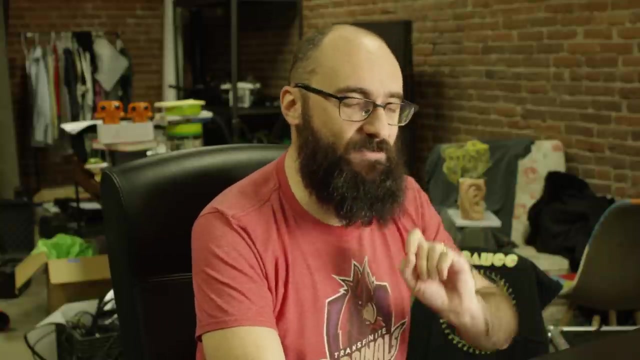 going to need nine more b's. We already have a c, so we don't need to add any more c's. There you go. This right here is equal to this: the actual amount represented by the original number- Oh, look at this, This is very interesting- 99a plus 9b- This part of the expression. 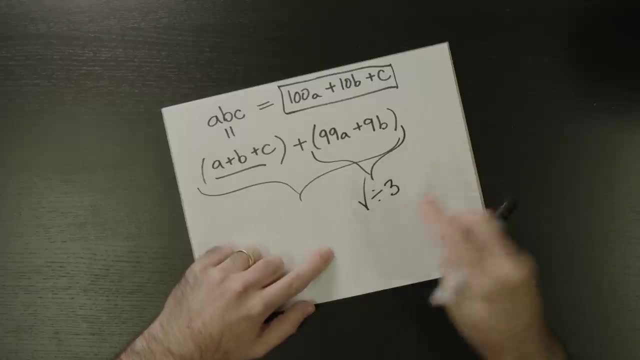 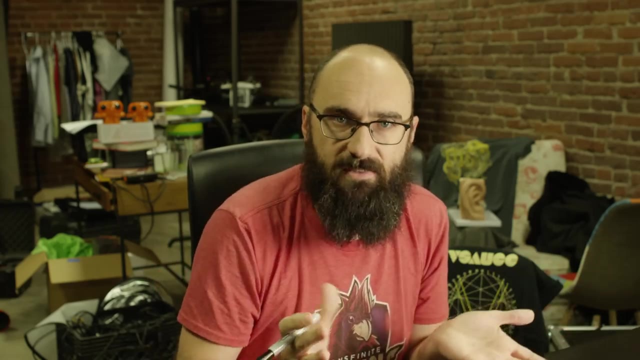 will always be evenly divisible by three, No matter how many digits are in the number that you are checking. every coefficient in this part will just be a string of nines, which means each term in it will be divisible by three. And if you add a bunch of groups of three to another bunch of 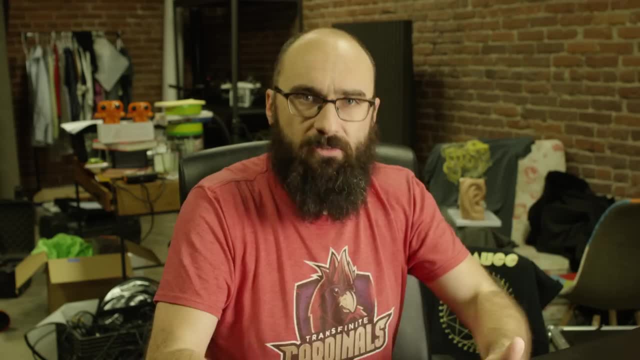 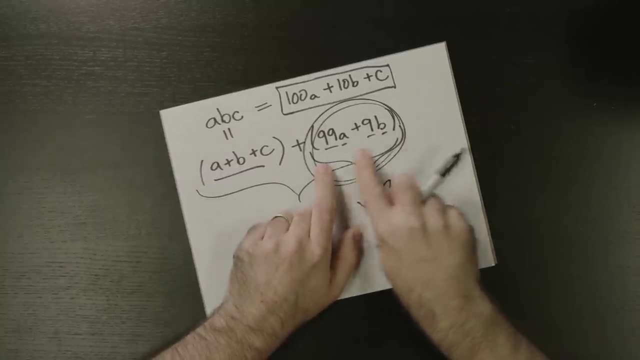 groups of three. well, what you're left with is just a bunch of groups of three. What you're left with is a sum that is still divisible by three, And so, because this component is always divisible by three, all we need to do is divide it by three, And so, because this component is always divisible, 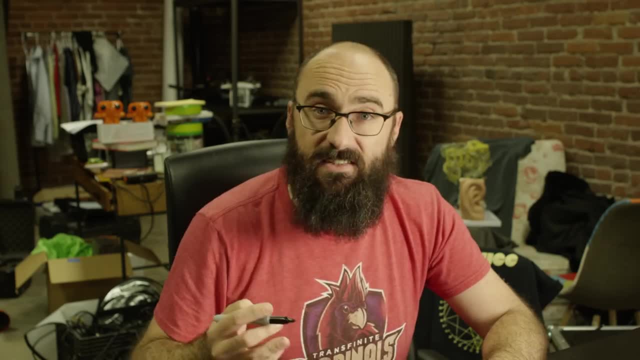 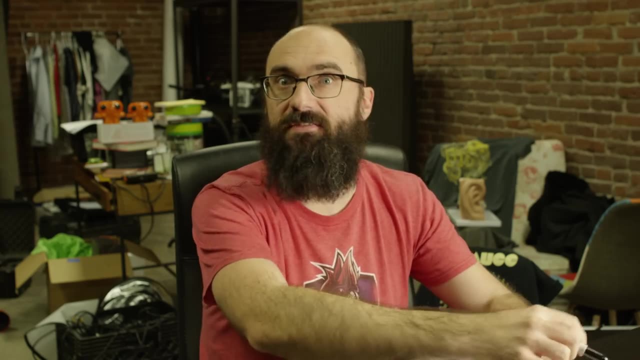 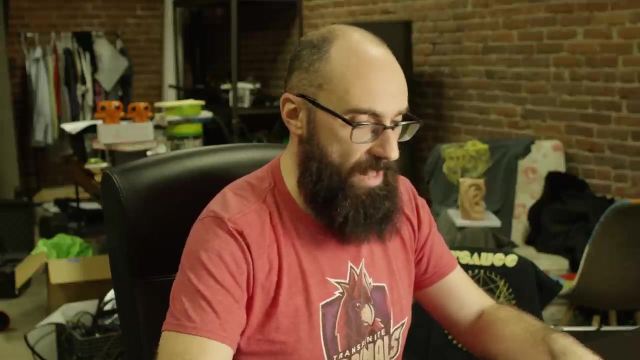 by three. all we need to do is check whether this part is. If it is well, then the original number is the sum of two numbers divisible by three, So it itself will be divisible by three. In a similar way, the divisibility check for four operates as well, So let's. 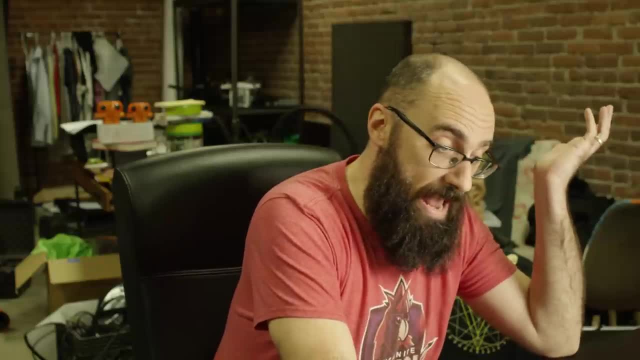 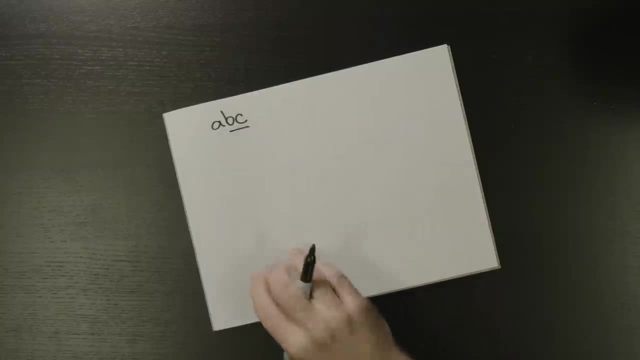 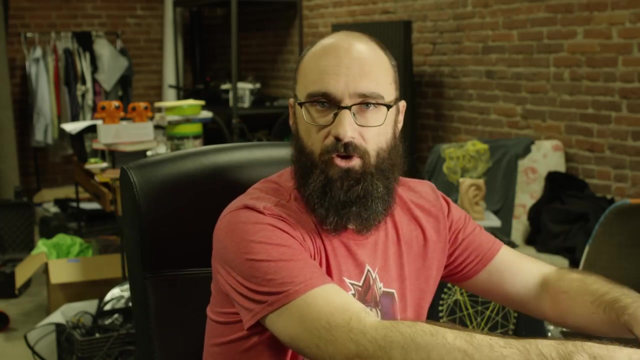 check that. Let's again say that we have a number like a and b and c. Now remember that when we checked for divisibility by four, we only concerned ourselves with the last two digits. Why would that be? Well, it is because, conveniently, four goes into one hundred, an integer number. 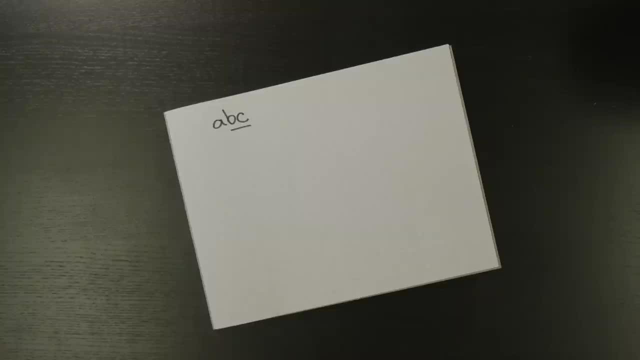 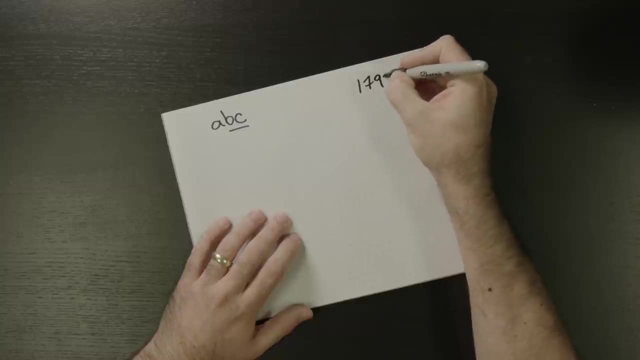 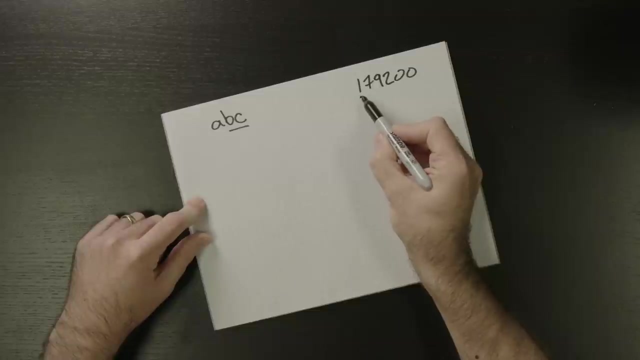 of times Twenty-five in fact. So any number that ends with at least two zeros is divisible by four. For example, the number, let's say, one, seven, nine, two, zero, zero. I just made this one up, But I know that four will evenly go into this, because it is just one thousand. 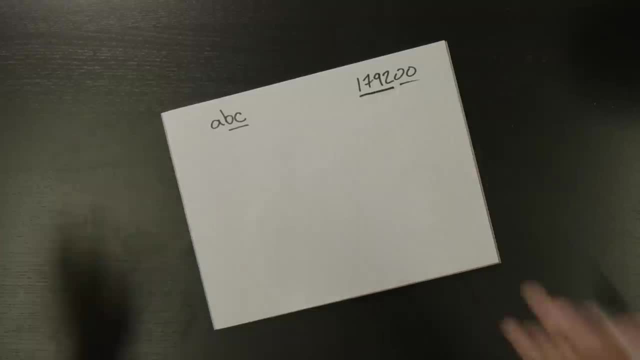 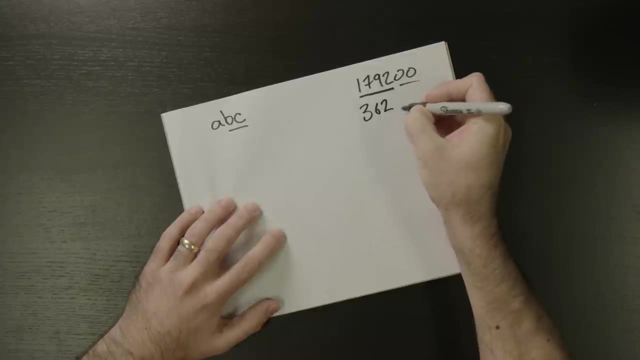 seven hundred and ninety-two hundreds, And four will go into one hundred and twenty-five, And four goes into a hundred. What that means is that when we take a number like the number that we started with, 362 thousand eight hundred and eighty, it doesn't end with two zeros. 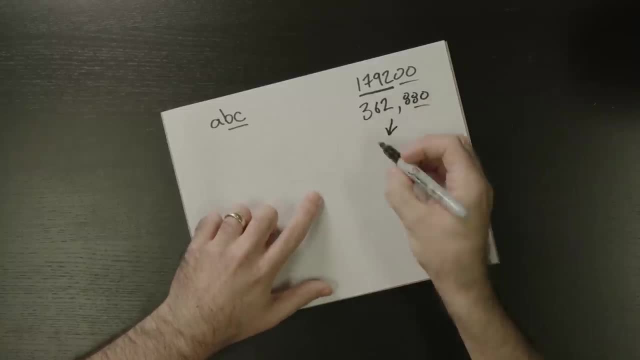 but we can think of it as being, uh, three hundred and sixty-two thousand eight hundred, which we know that four goes into plus eighty. So we only need to check the divisibility of this component, those last two digits: eighty Five. 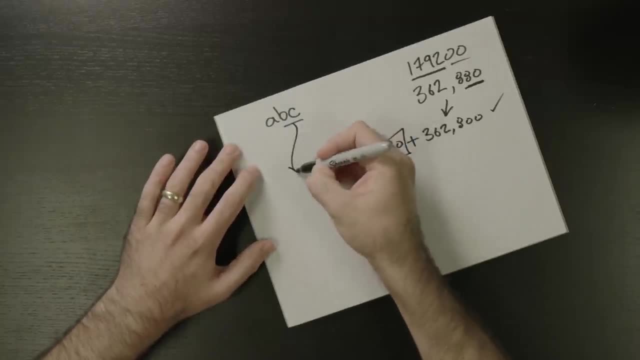 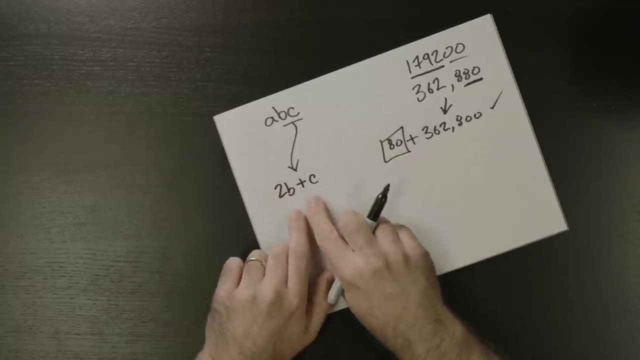 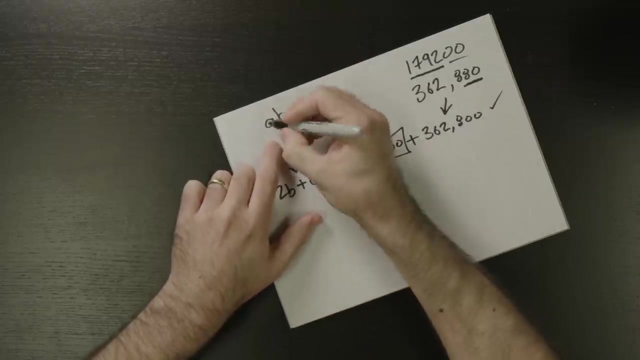 Five Eight, All right. so remember, we took BC right. We took the last two digits and we doubled the tens digit and then we added the ones digit. Why does this work? Well, in the same way that the check for divisibility by three works. let's remember that BC. we're forgetting about A for now. 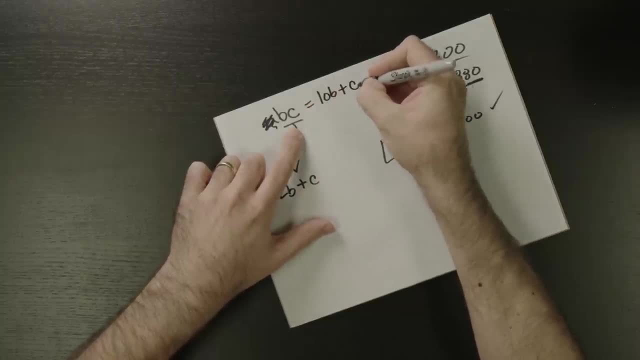 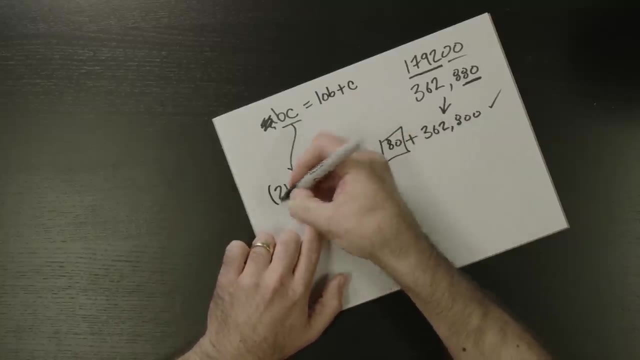 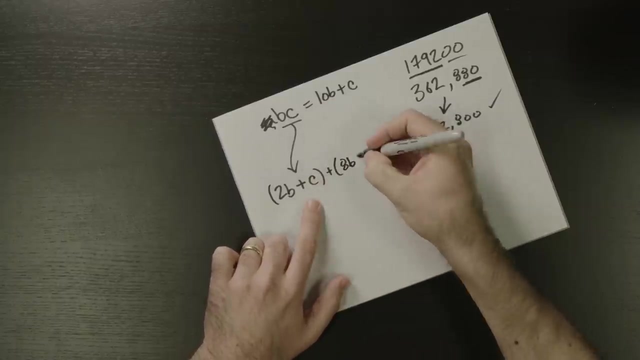 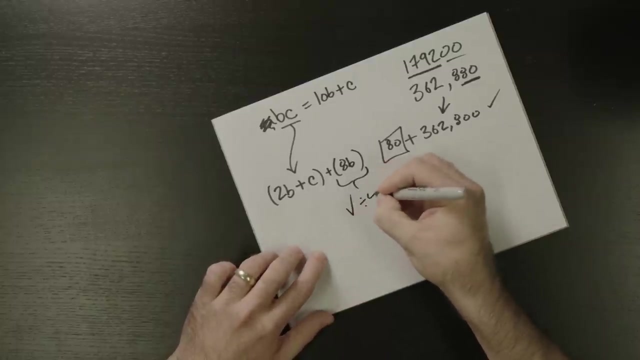 BC means 10 times B plus C number of things. Well, how do we get from this checking expression to the actual value of BC? Well, we're going to need eight more Bs and no Cs. Well, look at that. eight, eight B, eight B will always be divisible by four because eight can be put into groups of four. 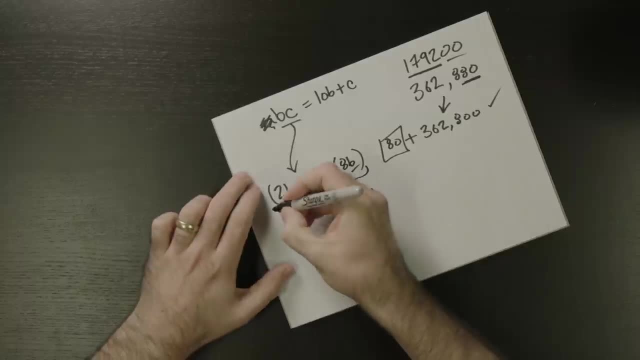 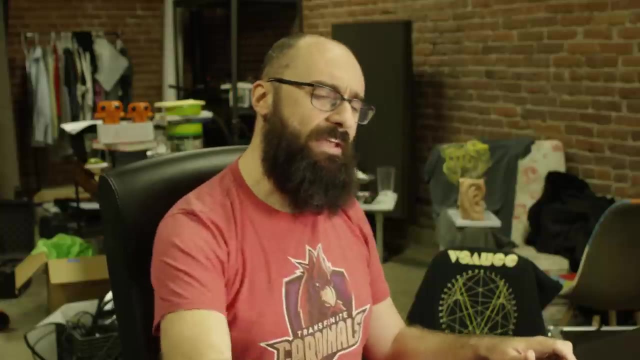 and we're going to have B times as many of those groups of four. so we only need to know if this other part is divisible by four, and if it is well, then The entire number is. You might think, oh well, why don't we just use this trick to check for divisibility by eight? 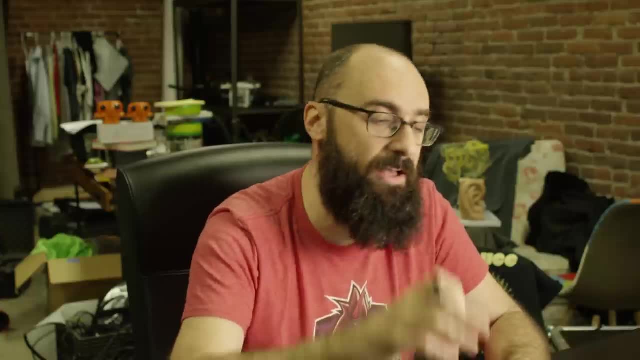 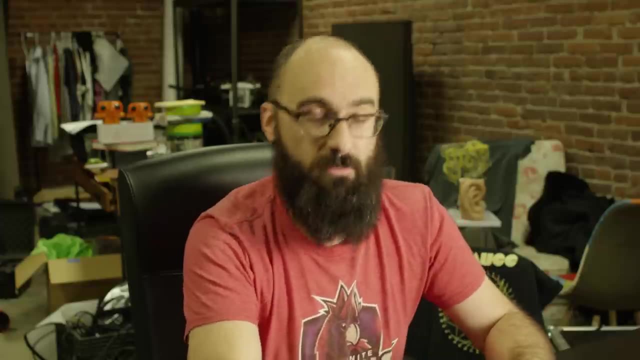 I wish that we could, but the problem is that this entire trick relies on the fact that the last two digits of the number are all that matter, because four goes into 100, but eight does not. However, eight does go into 1,000. 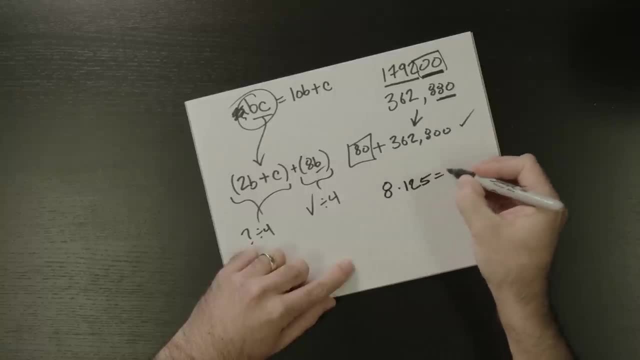 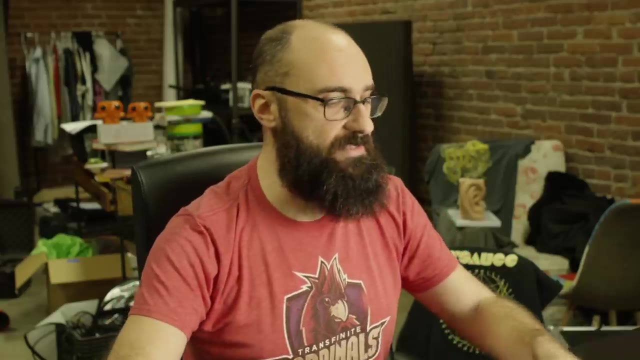 Eight times 125 equals 1,000. So if a number is, If a number ends with three zeros or more, we know that it is evenly divisible by eight. We only need to worry, then, about the last three digits of any number to check for divisibility by eight. 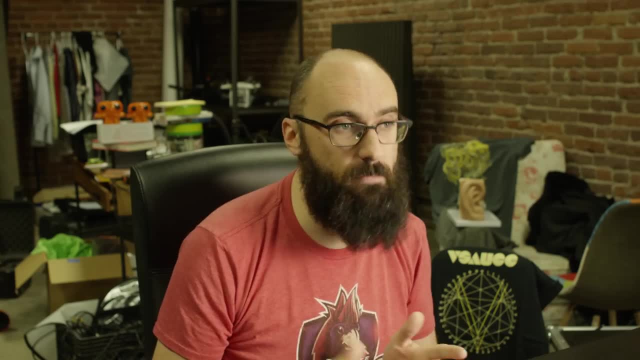 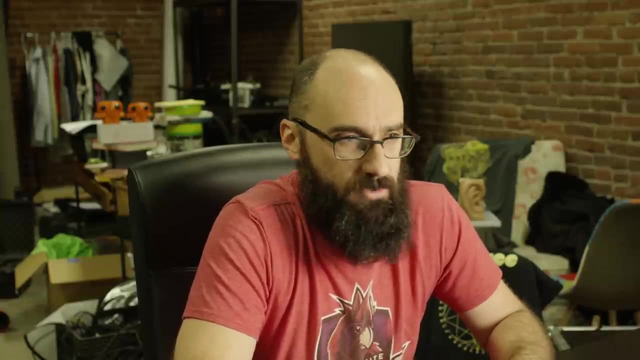 If you're thinking about a number that doesn't have three digits, that's only a two-digit number, well then you know, you probably can just figure out if it's divisible by eight by simply knowing your eight times tables. If you know them, if you've memorized them up to eight times ten at least, well, that's already 80.. 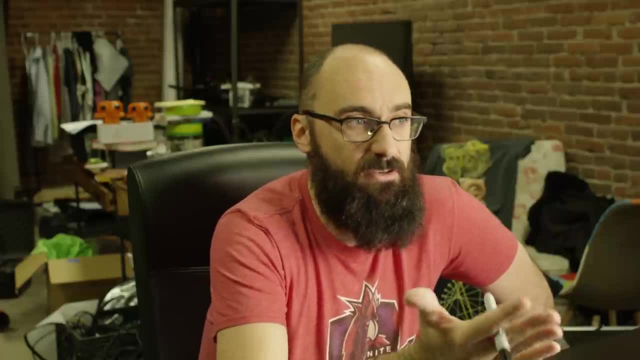 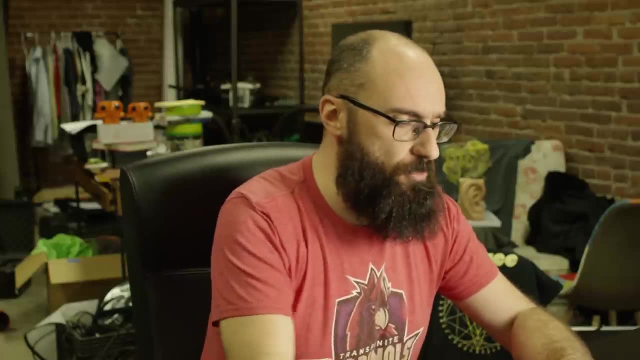 From there you go from 80 to 88, and then you go to 96. And then you're done. Those are the only other two-digit multiples of eight. 96 is eight times 12,, of course, But when it comes to a three-digit number I'll say ABC. it doesn't matter what other digits are out here, if any. 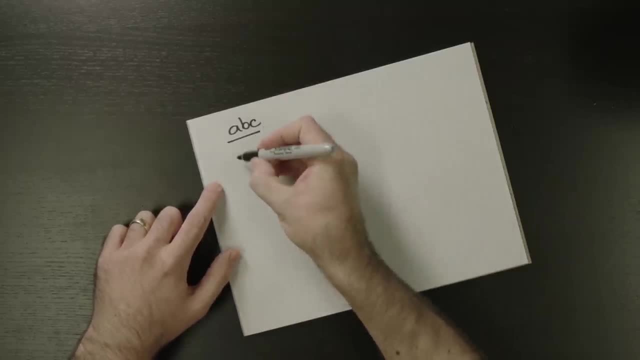 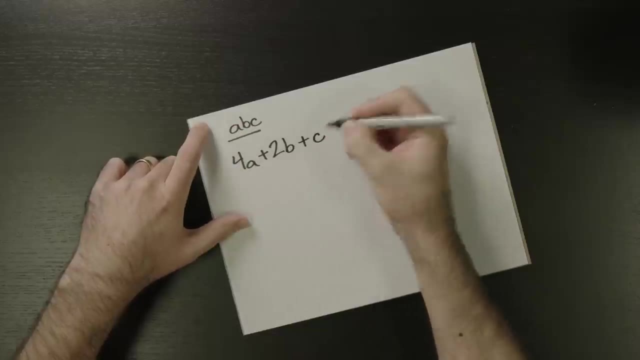 We check divisibility by eight by taking four times the 100's digit and summing that with two times the 10's digit and then just the unit's digit by itself. Why does this allow us to check for divisibility by eight? Well, let's take a look. 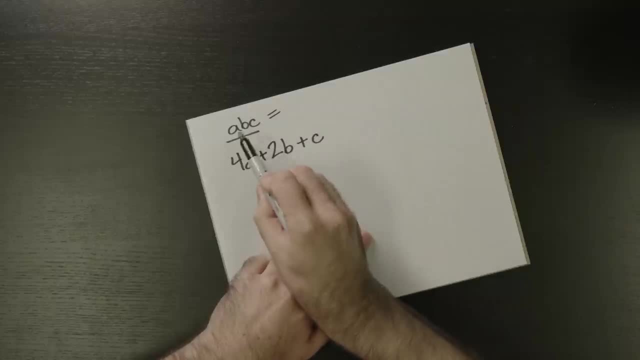 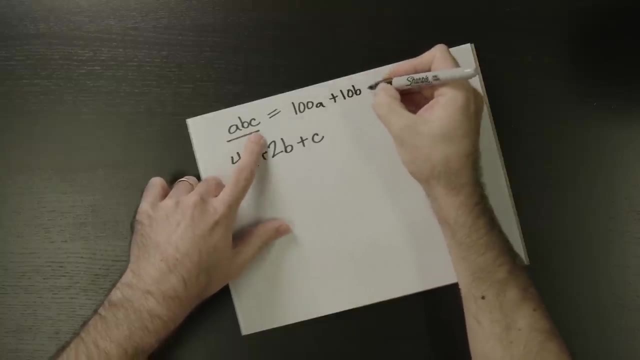 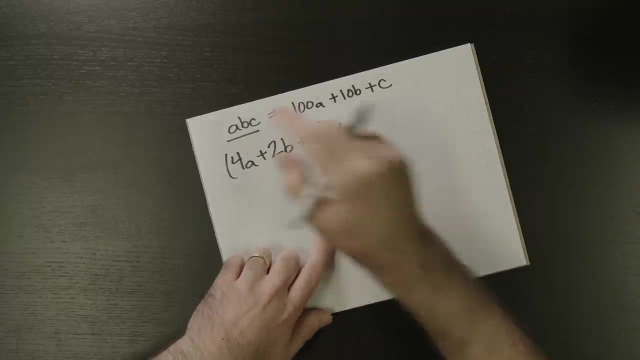 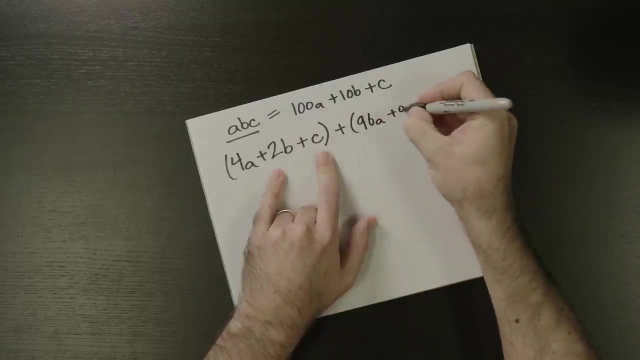 We know that the actual amount represented by ABC is equal to 100 times A plus 10 times B plus C. To get from this expression, the checking expression, to the actual amount represented by ABC, we need 96 more A's, we need eight more B's and no more C's. 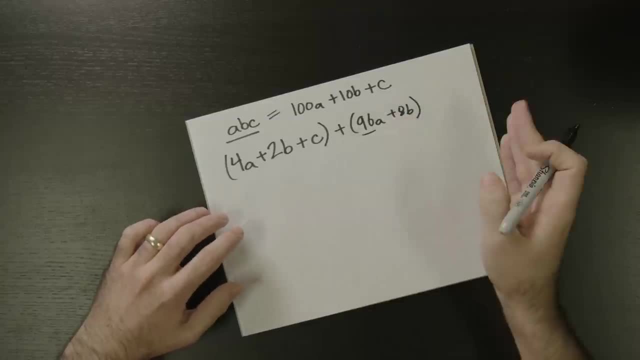 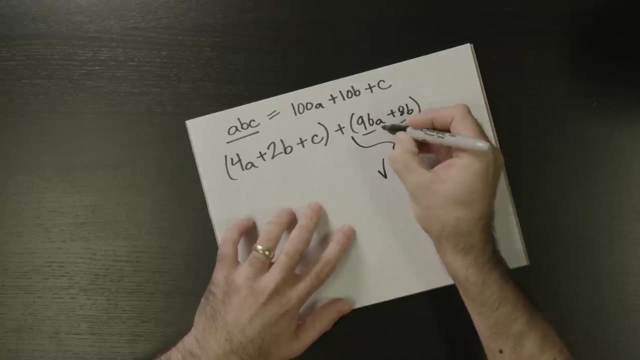 Well, we just talked about how 96 is eight times 12.. 96 is eight times 12. And, of course, eight goes into eight. So this part is always divisible by eight, regardless of what A and B are. So we only need to make sure that this expression is divisible by eight. 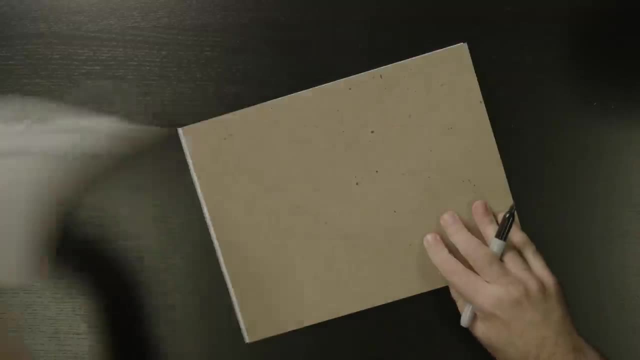 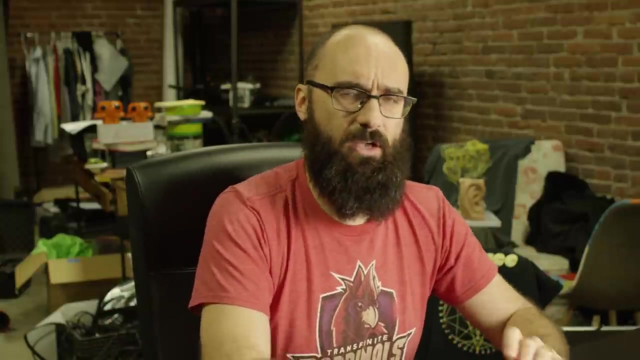 If it is, then the original number is Okay. You know what? All we have left to discuss now is divisibility by seven. Why did that trick work? It was kind of strange. right, We took the one's digit of the number, multiplied it by five and then added it to the number. 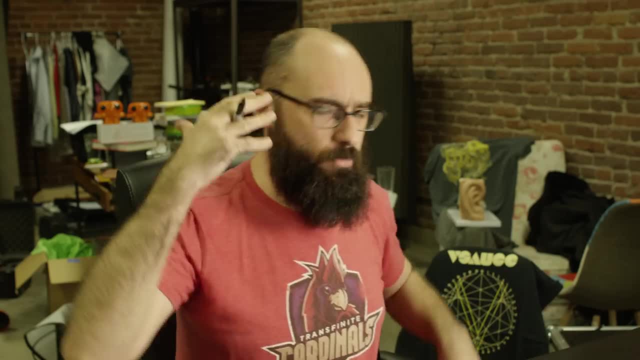 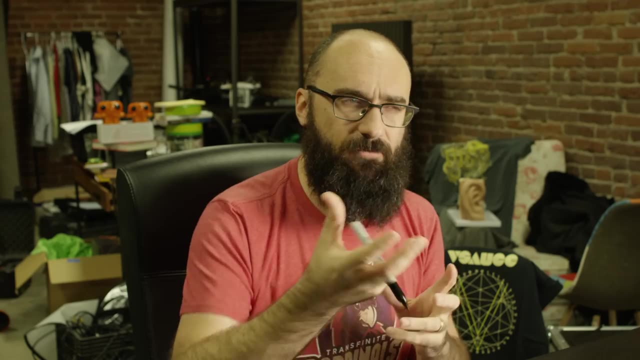 And then added it to what was left. Well, the trick to kind of wrapping your head around why this works is to figure out what it means to sum what's left after removing the one's digit. So let's say that we have a number like ABC. 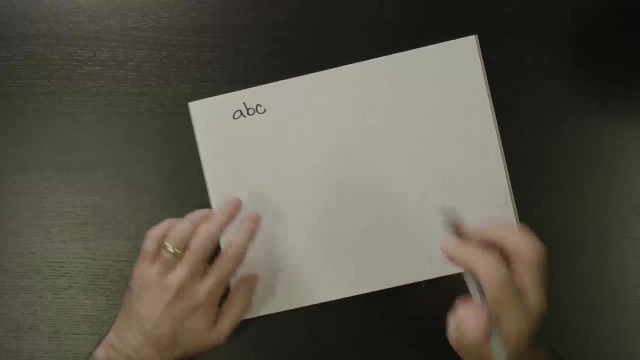 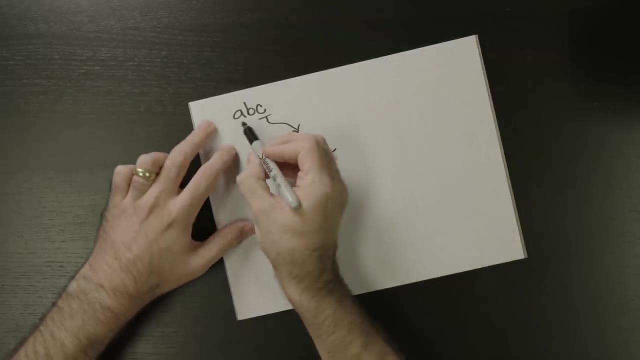 It doesn't have to be three digits long, You could do it of any length. But we take this one's digit, C, and we multiply it by five And we add that to what's left. How do we represent this procedure of taking what's left? 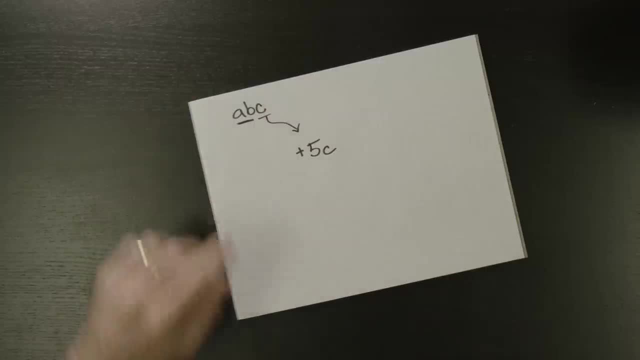 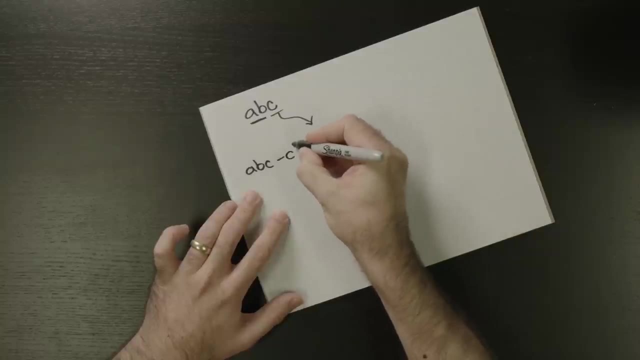 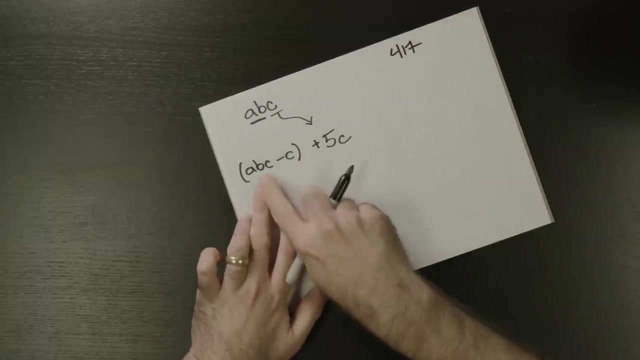 And treating it like it's its own number. Well, one way to do that is to think about the original number, ABC, and then subtract C from it. Okay, This would allow us to take a number like 417 and then subtract that last digit, seven. 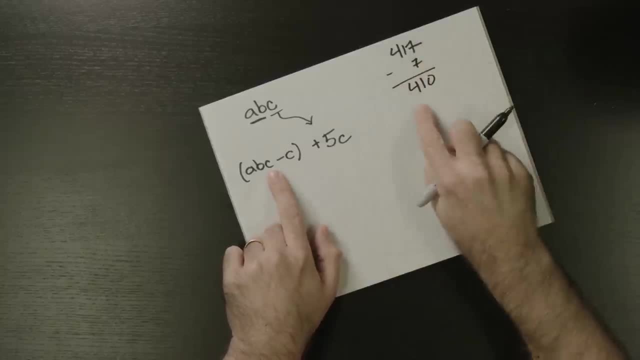 If we subtract seven, then we're left with 410.. We've turned the one's digit into a zero. Then we want to just get rid of it completely, And we can easily do that by dividing by 10, in which case we then wind up with 41. 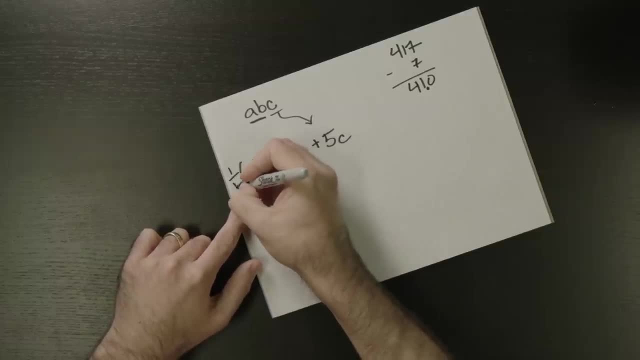 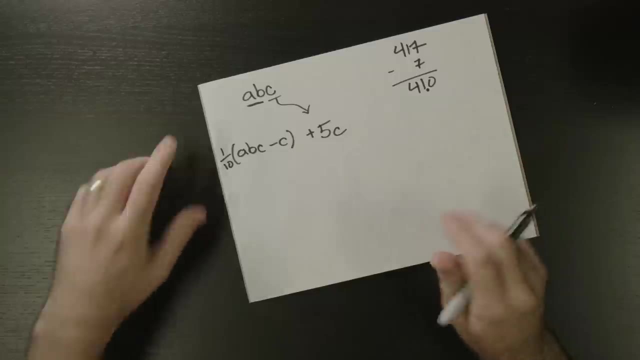 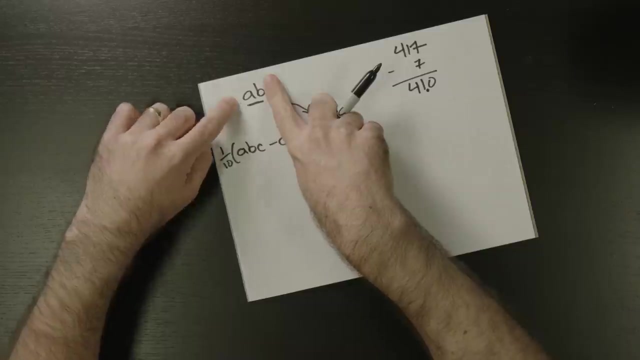 So we're going to have to divide this by 10, which is the same as multiplying by 1 tenth. This looks a little bit messy And I hope you're able to follow it. All we're trying to do is algebraically show what is done when we ignore the one's digit and treat what's left as its own number. 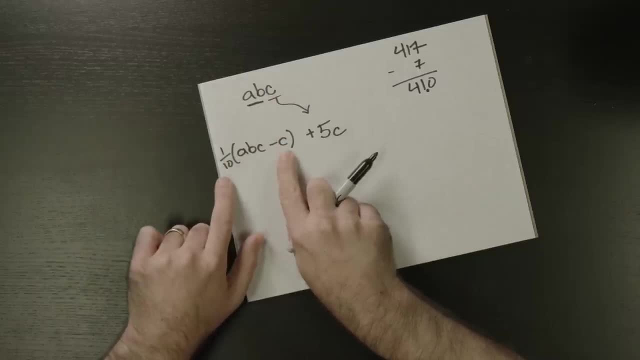 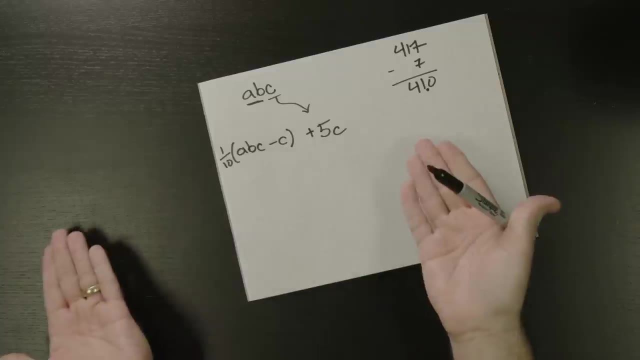 That's what we're doing here. We're taking away the one's digit, so it becomes a zero, And then dividing by 10.. So we turn ABC into just ABC, Perfect. Now how does this, and whether it's divisible by seven tell us that this is also the original number is also divisible by seven. 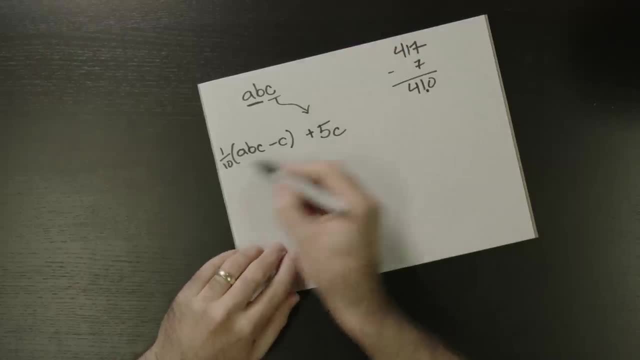 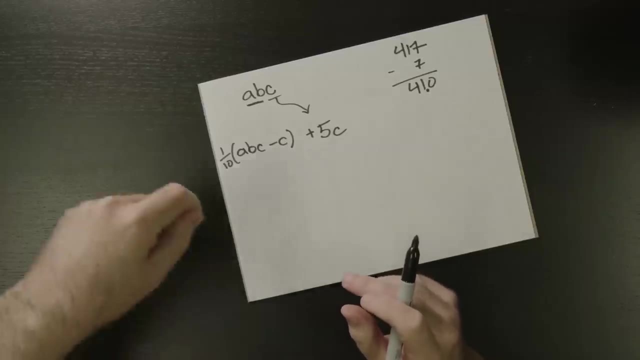 Oh boy. Well, this is very fun. Let's play around with this expression and see what else it is either equal to or divisible by the same numbers as Okay. So let's distribute the 1 tenth first, Because 1 tenth times this stuff, in parentheses, can also be represented as a zero. 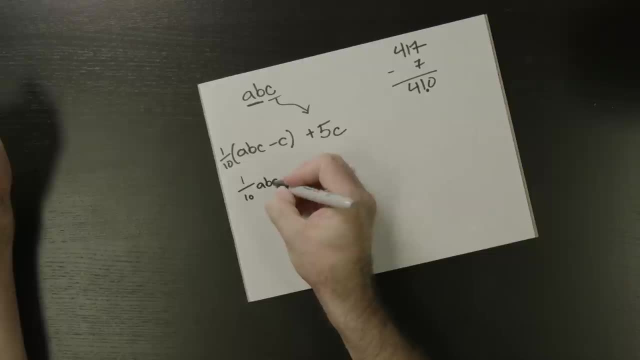 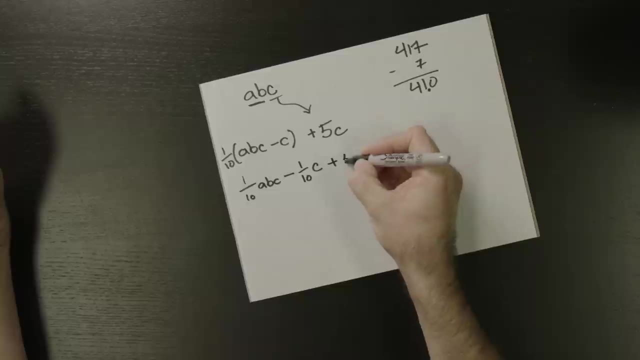 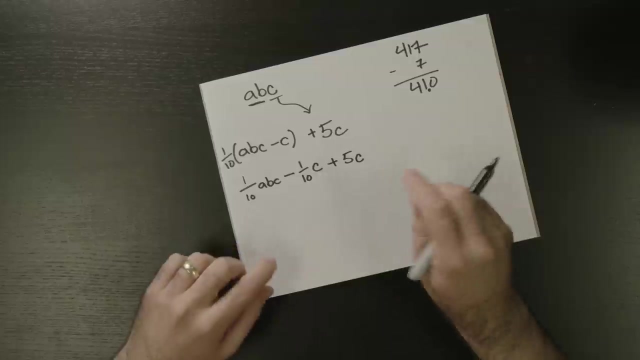 Or it can be represented as 1 tenth times ABC minus 1 tenth times C. All right, And we still have to add the 5C at the end. Oh, look at this, We've got ourselves two different amounts of C. 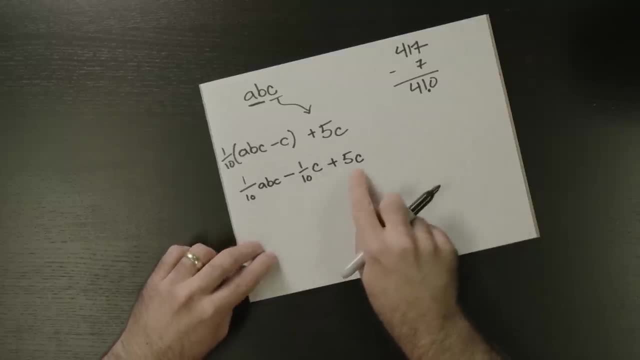 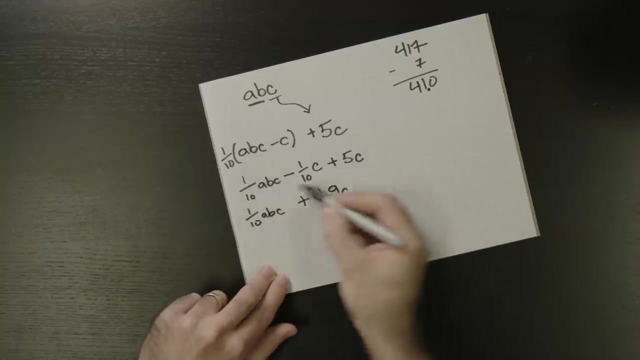 We can combine those. What is 5C minus 1 tenth of a C? Well, that's 5 minus 0.1.. 5 minus 0.1 is a positive 4.9.. still have this 1 tenth ABC. So this expression right here, this third one that we've got. 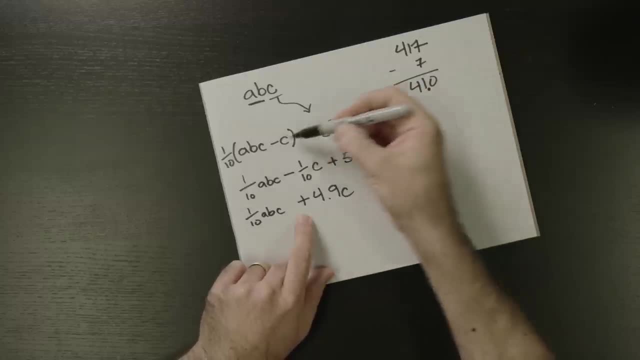 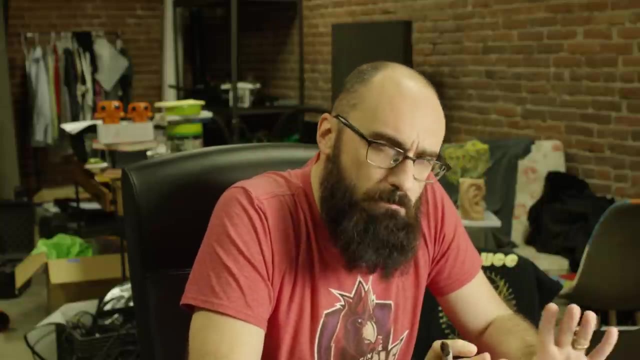 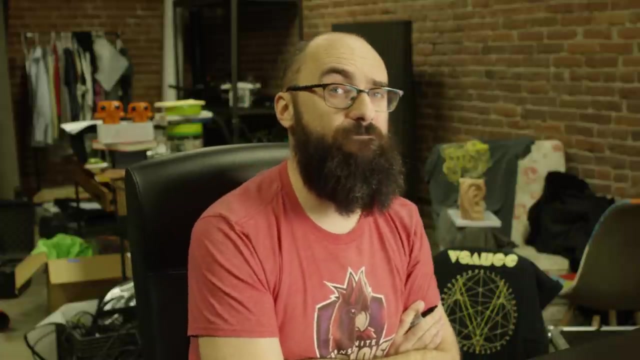 is equal to this expression, which is equal to this expression that we actually are using to check for divisibility by 7.. You might already have a bit of a sense of why this works, because 4.9 looks an awful lot like 49,, a number that is famously divisible by. 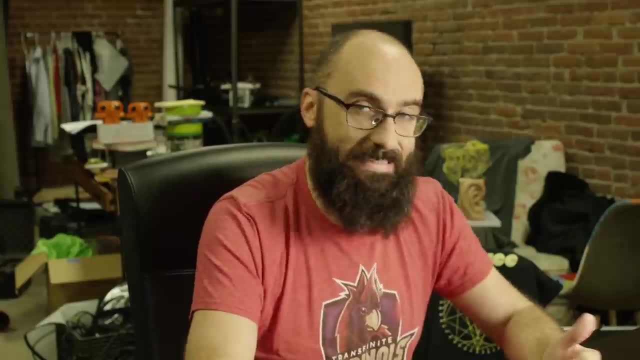 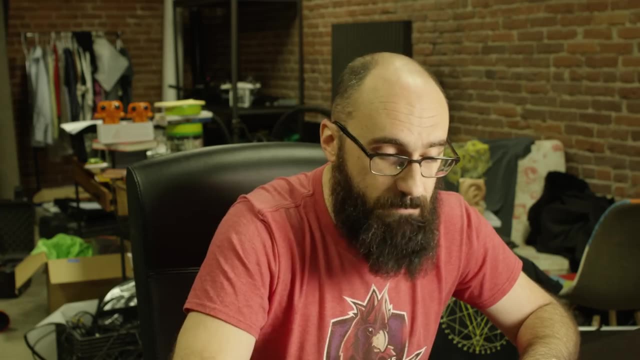 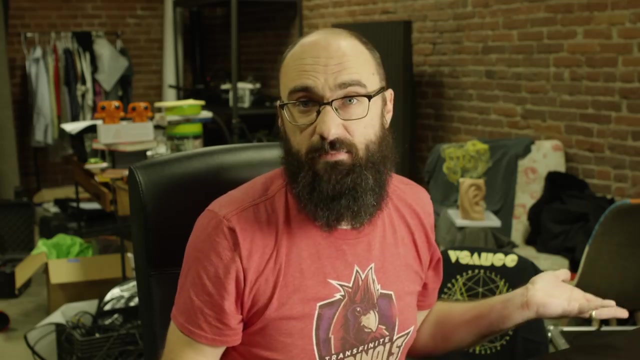 7. Let's go ahead and make this even easier by taking this and multiplying it by 10.. Multiplying by 10 doesn't change what this can be evenly divided by. It just means that whatever amount of groups we can make, we're going to have 10 times more of them, right? 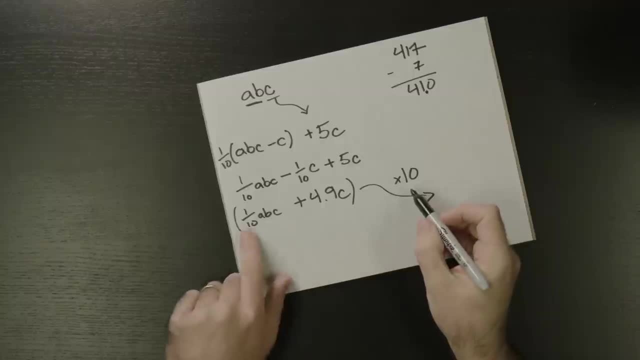 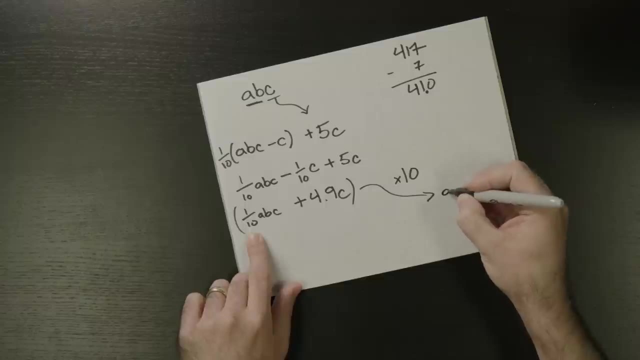 It doesn't add any remainders. so we're fine. If we multiply this whole thing by 10, that means we're multiplying 1 tenth ABC by 10.. 10 times 1 tenth is 1, so we've got a big. 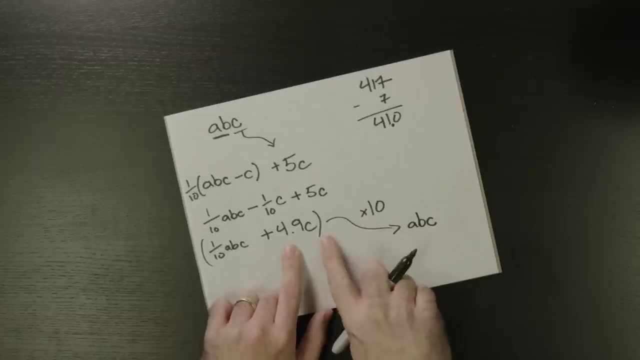 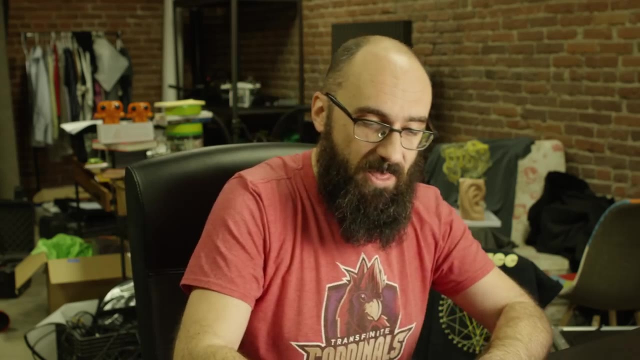 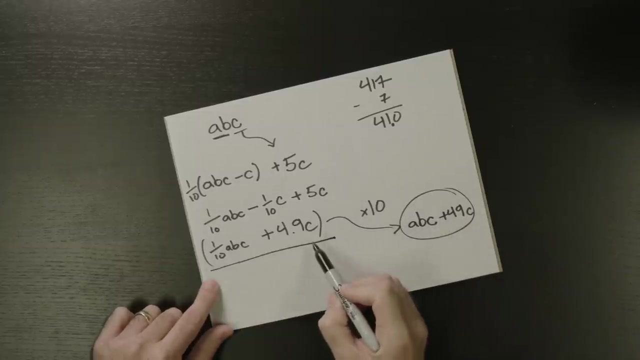 C, And then 10 times 4.9, well, that's just 49C. Oh, look at this. Alright, so this thing that we've wound up with is divisible by the same numbers as this, which is divisible by: 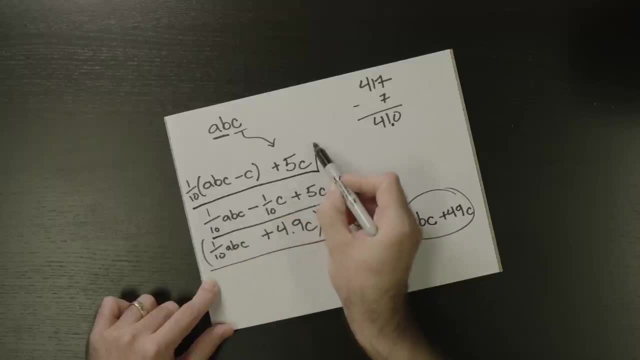 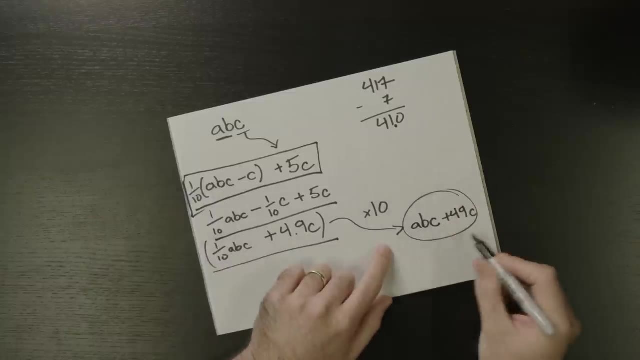 the same numbers as this, which is divisible by the same numbers as this: the actual procedure we use to check for divisibility by 7.. But look at this guy. This is divisible by the same numbers as this. 49C is pretty clearly made up of a part that is always going to. 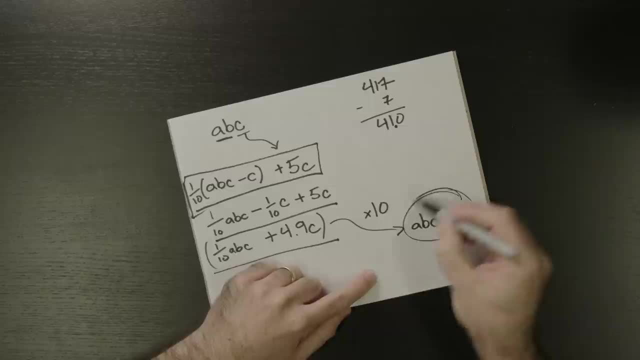 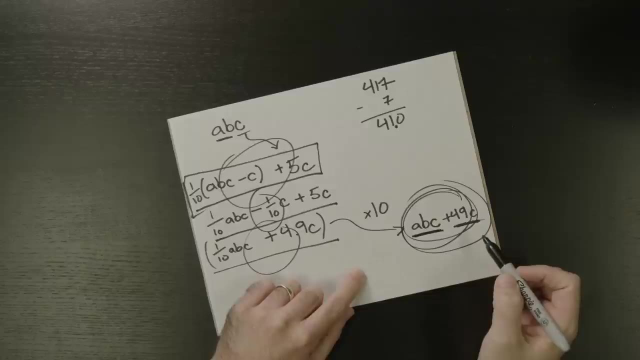 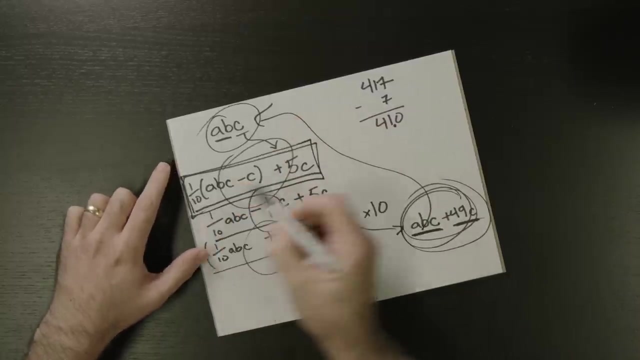 be divisible by 7.. 49 things can be put into groups of 7, and we're going to have C times more of those groups. So if this, if this, if this and if this happen to be divisible by 7,, well then that means that ABC must be 2.. But ABC is the original number. So if 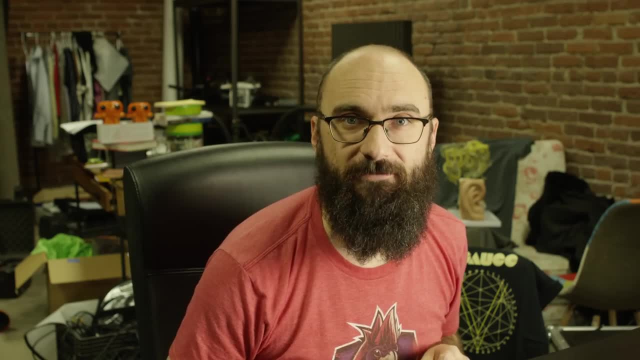 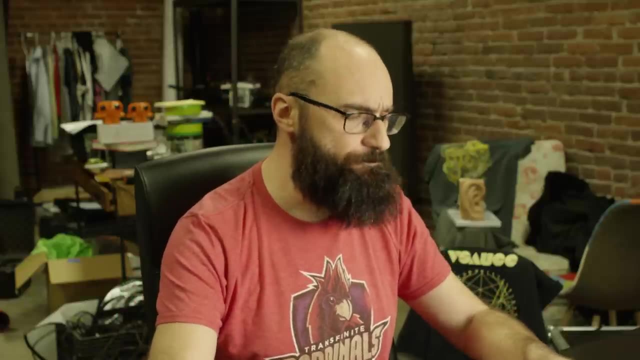 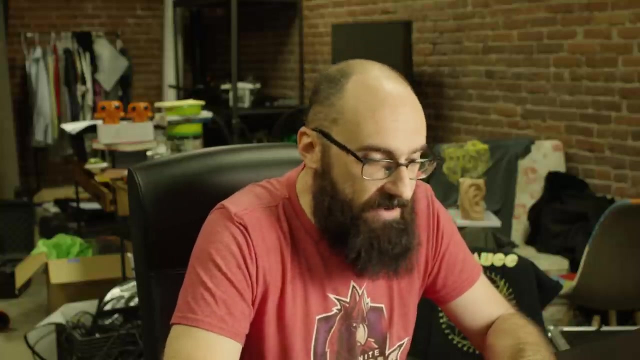 number we started with was two. Beautiful. I love this kind of stuff. If you've got some time while you're quarantined, I highly recommend playing around with numbers and coming up with some of your own tests of divisibility. It's very fun. I did it for six and I loved it. Obviously, 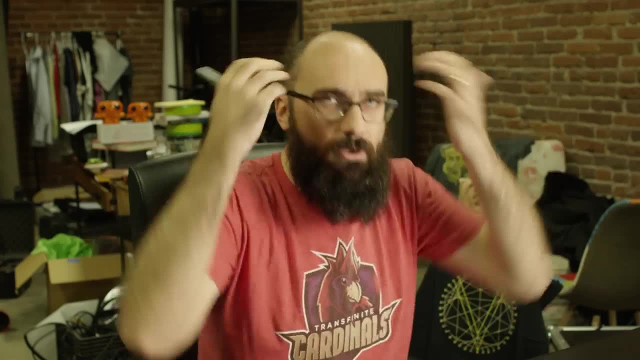 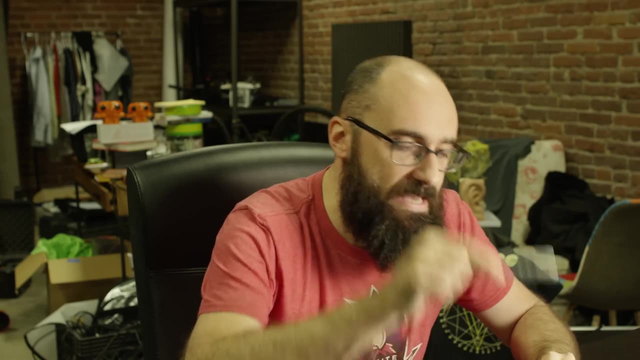 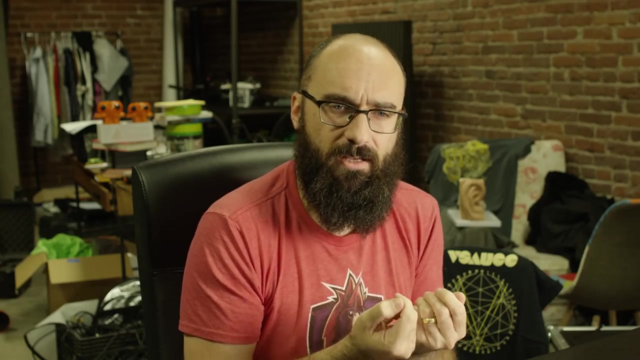 this doesn't necessarily make math faster to do. A calculator will be faster almost all the time, except if you've memorized things. But the point isn't speed. The point of these exercises is to develop our number sense and come closer to this thing we call number. 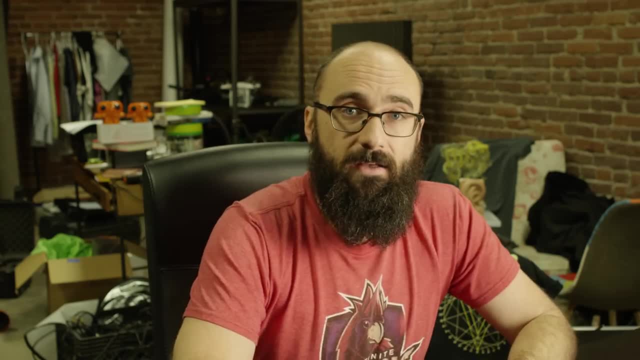 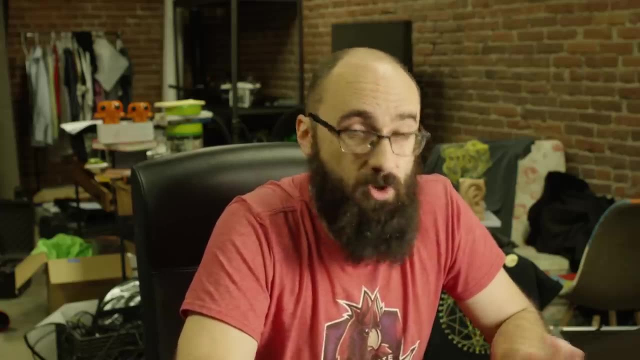 Now I'd like to end with a word from our sponsor, Vsauce. Those of you who subscribe to the Curiosity Box, thank you, Thank you so very much. I hope you know how much your support helps us here at Vsauce And, in my opinion, I hope you know how much your support helps us here at 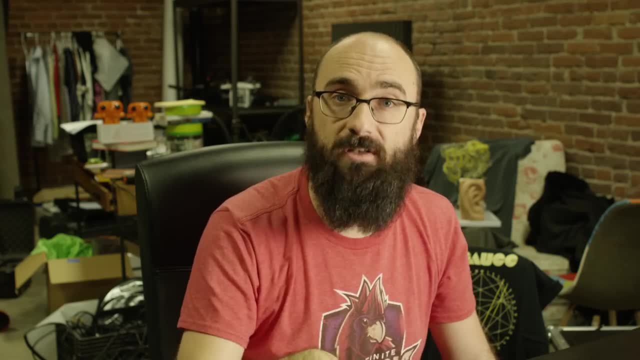 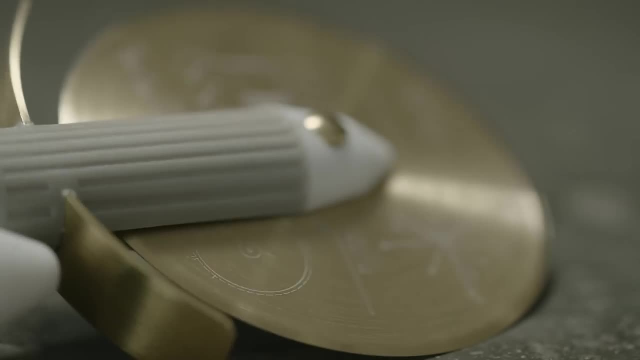 Vsauce And, in my opinion, helps make the world a better place. It's because of your support that we are able to make things that otherwise wouldn't exist, And they are things that I am very proud of, things that I'm glad for the world to have. The latest box- oh, I'm just thrilled. 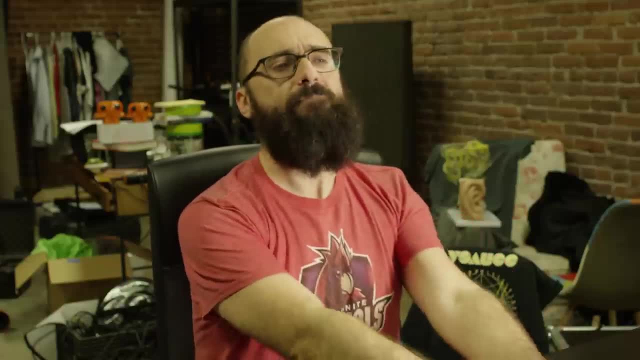 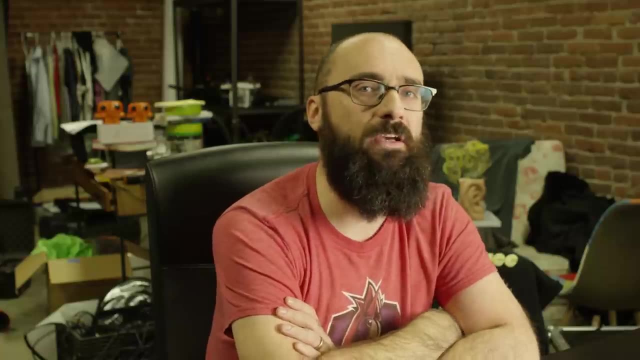 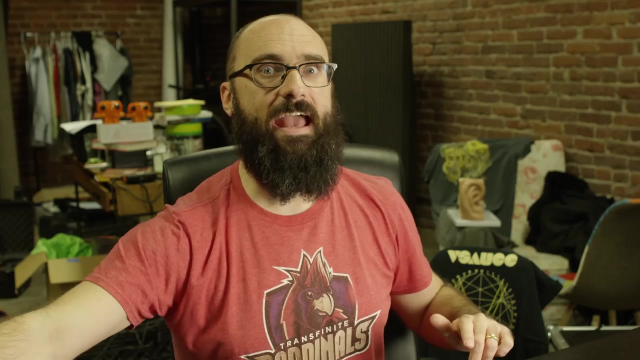 with something that we were able to make and include in it. In 1933, Theodore Edison, son of Thomas Edison, invented a puzzle that he called the Calibron 12.. And we went back to the original, Took the measurements and created a replica of the Calibron 12.. Look at that. 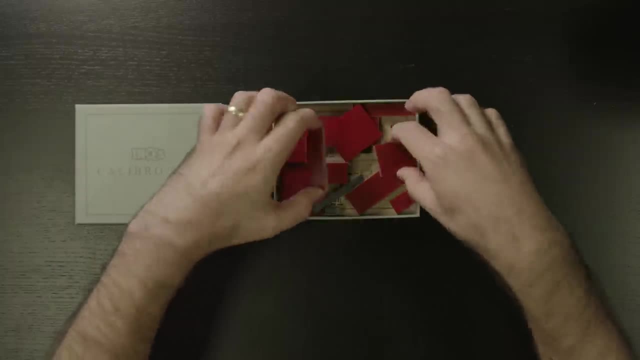 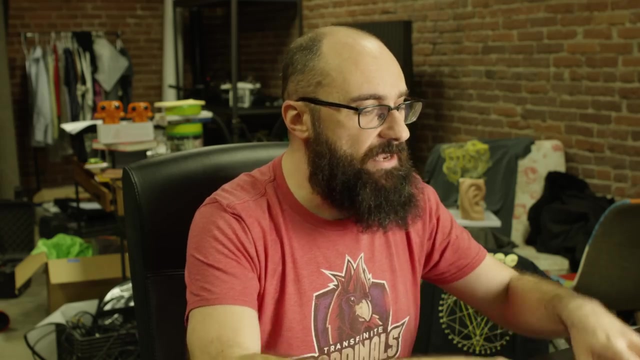 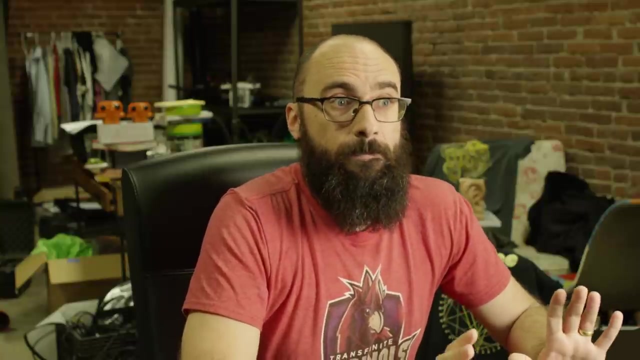 Very beautiful. The pieces are all of the same size as the original and they're even made of the original material: Bakelite. Now I'm excited about this puzzle because it is- I'm being totally serious- it is the only puzzle that I own that I have yet to solve. 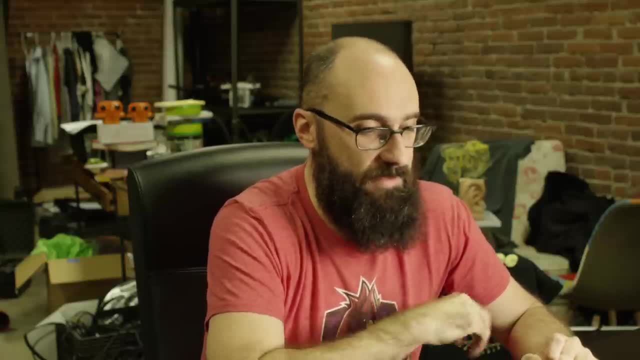 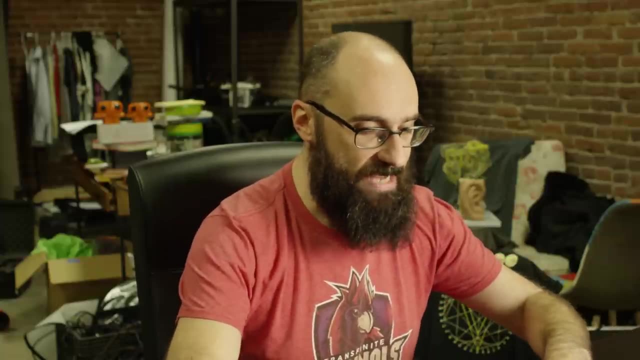 I have a wooden version of this puzzle that's a little bit different than the original and I've had it for a couple of years and I still have not figured it out. The puzzle goes like this: You take these 12 sort of burgundy pieces and you need to assemble them into a 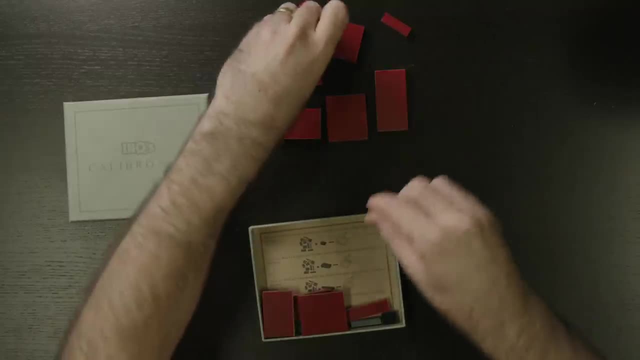 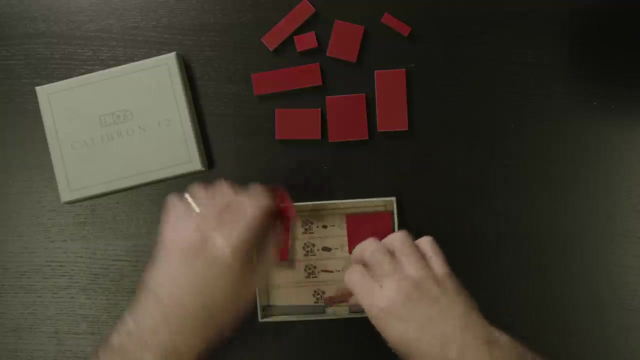 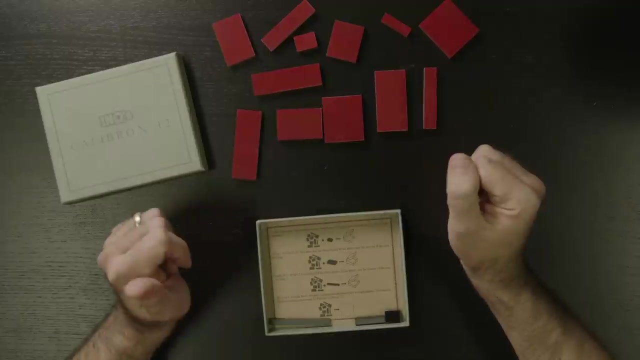 rectangle. That was the original puzzle. but the puzzle came in a box just like this And the pieces all came flat in the box. But this box's shape is not the shape of the rectangle that the 12 burgundy pieces fit into. 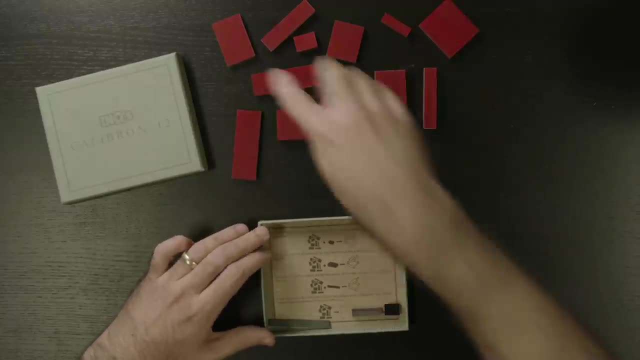 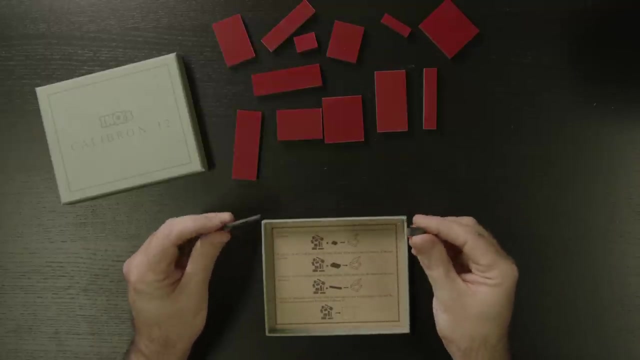 This is a different dimensioned rectangle, and in order to make these 12 pieces fit into here, you need to use one of these three black pieces which Edison called spacers. So all 12 pieces came in the original box along with a spacer. 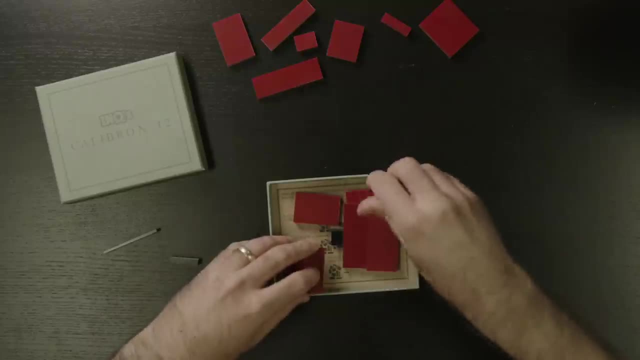 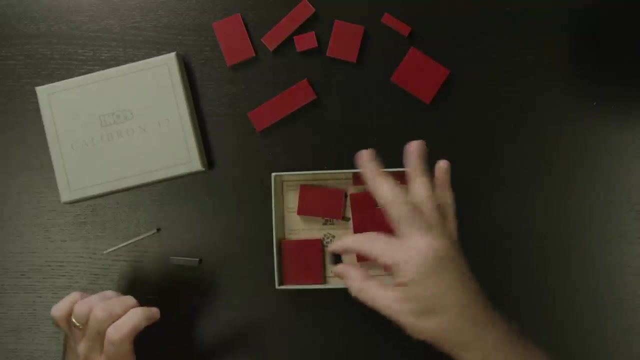 So it would be something like this: And somehow all 12 of these burgundy pieces and this 13th black spacer piece can be fit into the box. Once you've solved that puzzle, replace this spacer with a different spacer like this one, and now try to fit them all in. It's possible. 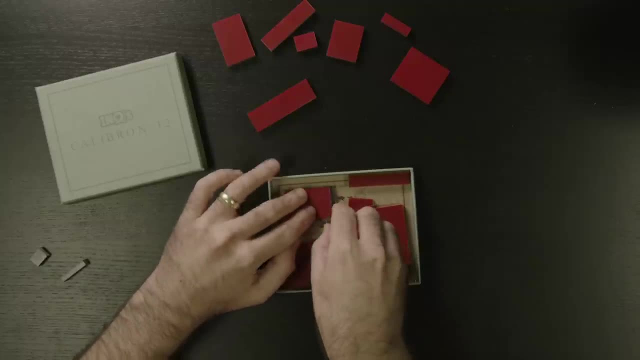 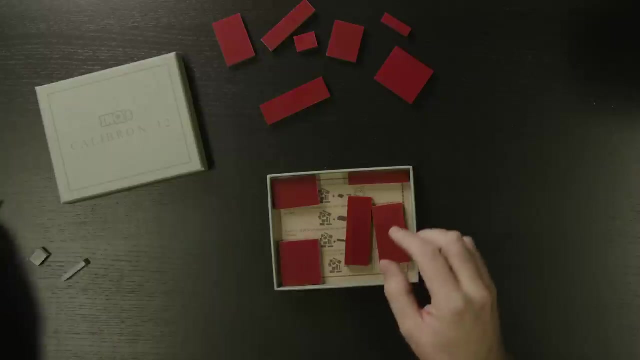 When you're done with that puzzle, then fit this nice little skinny dude in there and try to fit every piece into the box again. That's three different puzzles, but the original puzzle was just to take these 12 with no spacer and put them into a rectangle.